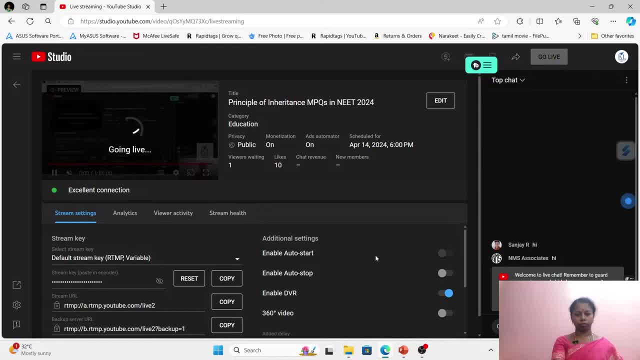 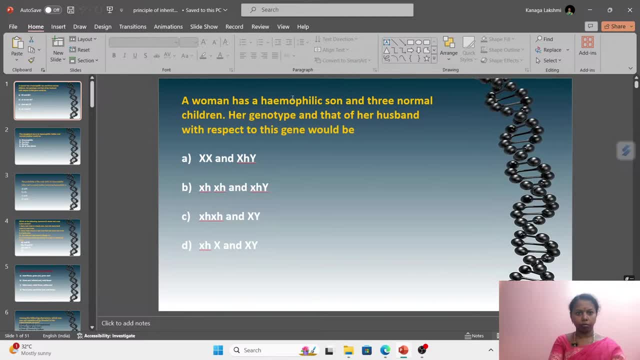 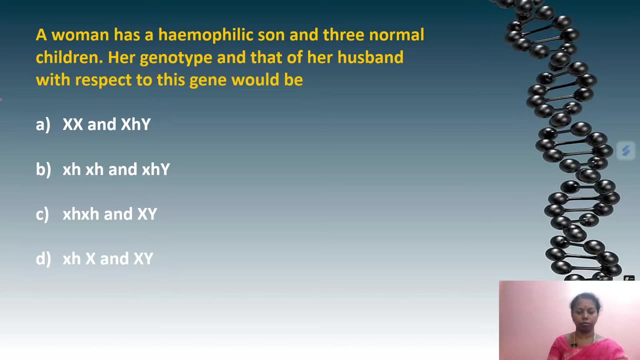 Thank you, Thank you, Thank you. Next question from this and these questions: sometimes it may be theoretical also, but sometimes we are getting like complication oriented questions. Okay, Check your skill. It's simply like probability oriented questions. they are asking children, So let us practice some probability oriented question to you all, as you were all asking, So it will be more helpful to you. how to face the questions of principle of inheritance in your NEET exam. 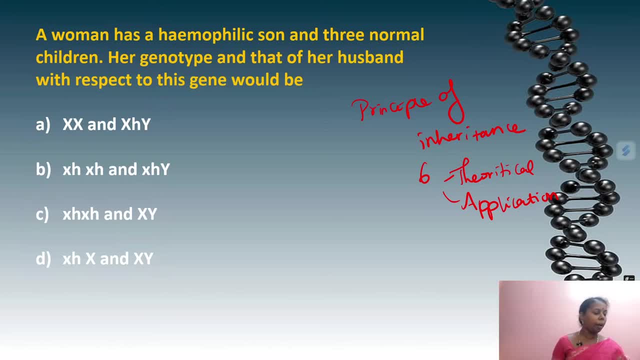 Yes, Dharani, Very good evening, Happy evening. Happy to see your name, So let us start the class. Yes, A woman asked, So next week I will be doing all your doubt sessions. So any topic, any question, if you are having doubt, you can send it to me directly in the comment box or in the WhatsApp number. what is given in the channel, so that we can discuss the questions there. Okay, 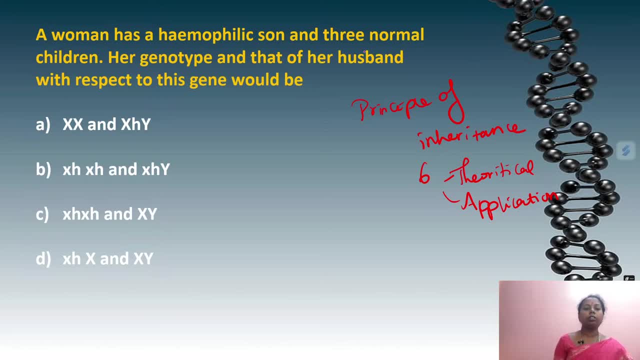 Okay, So you women? A woman has hemophilic sand and three normal children have genotype, and that of her husband with respect to this gene would be dash. Yes, Nandika, Very good evening. Yes, Dharani, Very good evening. We just started Dharani about principle of inheritance. We will be discussing all application oriented questions today. 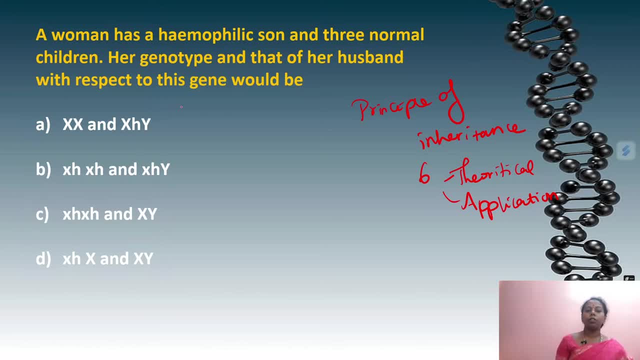 Okay, It will be more interesting and helpful also for you. The first question is: a woman has hemophilic sand. So she has a hemophilic sand- Okay, This is sand- and three normal children. So children are other normal. Her genotype and that of her husband would be. So woman is having the problem means hemophilic. So mother might be the carrier, Yes, And the father might be normal because the other children are normal. So the answer will be: 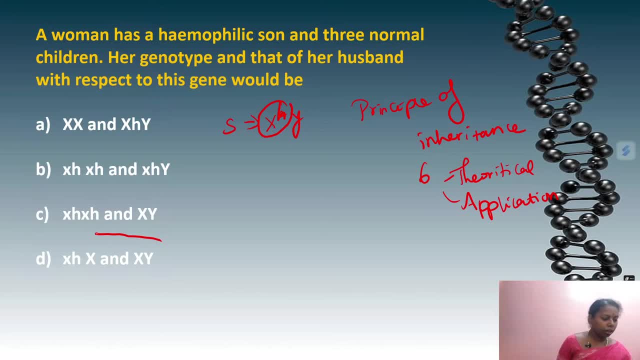 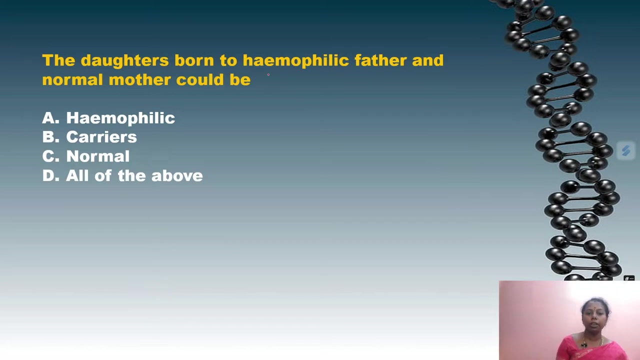 Yes, Lakshita, Very correct. Yes, Santosh, Very good evening. And yes, it is D. Excellent answer by you all. Yes, it is D, Of course, the mother is the carrier and father is normal. Okay, So now next question, Let us proceed. The daughter born to a hemophilic father and a normal mother. Okay, 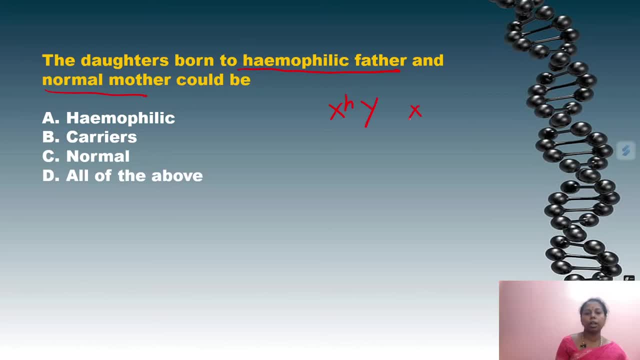 Hemophilic father. you know, it is the father's genotype: Normal mother, is what? X and X? So what about the daughters? they are asking: Can you try children? So what about the daughter? Father is hemophilic, but mother is normal. So in that case, what will be the condition of the daughters? Yes, Dharani, Excellent, They will be carrier. definitely XH and X. Okay, This is one Okay. 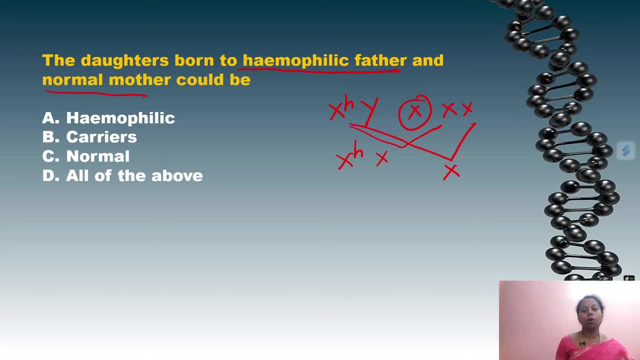 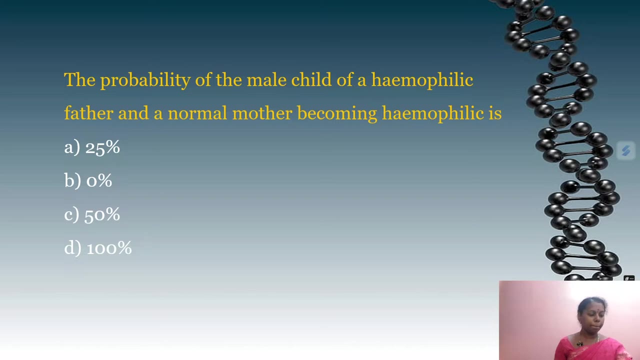 possibility or the other possibility also XH and X, So they are carriers. Is the correct answer? Excellent answer by Dharini. Very good, Dharini, Excellent, Okay, So let us proceed to the next question: The probability of male child of. 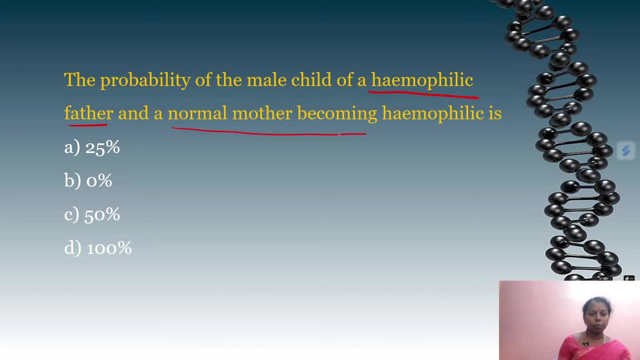 hemophilic father and a normal mother. So hemophilic father, X, H, Y Father. Okay, This is father, And of course the mother is normal means X and X Male child hemophilic. What is the probability They are asking? So can you try your answer: children? 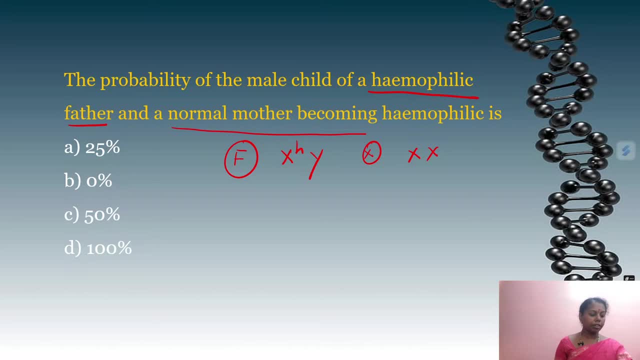 Yes, Again, Dharini has answered. It is B, Of course. Of course it is 0% Fine. So you know, for the male child, X is donated by the mother. So X, Y, X, Y is possible. Maybe for the daughter the father will donate. They will become carriers. 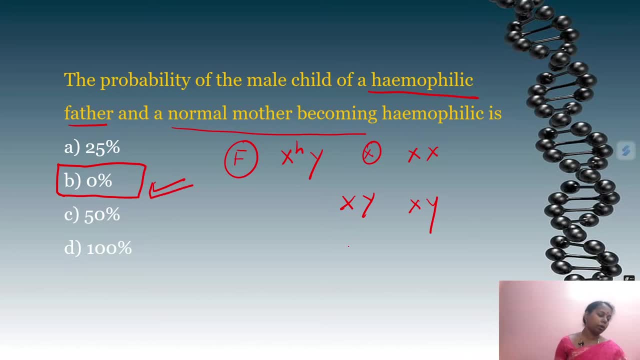 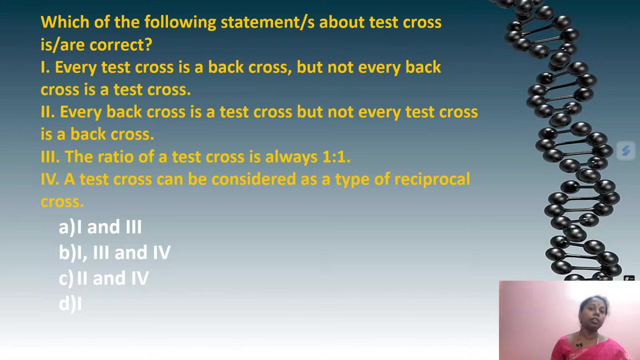 So for children, son will be 0% monthly. It is the very correct answer. Yes, Dharini, very correct, Okay. So keep taking your mark test. Take it correctly, Okay, And check your week's chapters Where you are doing wrong. 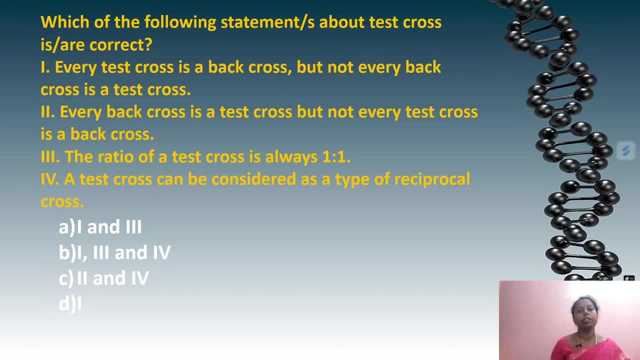 Are you doing it correctly in that chapter. You have to see that, And when there is a lot of mistake in that chapter and when it does not come, you can leave it in the choice. So don't crush yourself with the pressure. It is very easy. 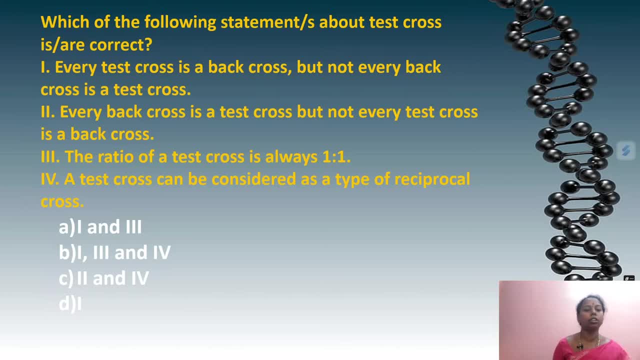 You can use your strong chapters. Okay, Let us proceed to the next question. Which of the following statement is about test cross or correct? Every test cross is a back cross, but not every back cross is a test cross. Every back cross is a test cross, but not every test cross is a back cross. 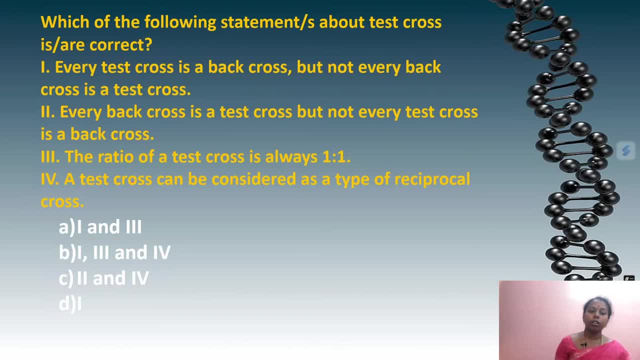 The ratio of test cross is always 1 is to 1.. A test cross can be considered as a type of reciprocal cross. So among this, which are all correct, is the question: Yes, Jeevan. Very good evening. Happy Tamil New Year, Jeevan. 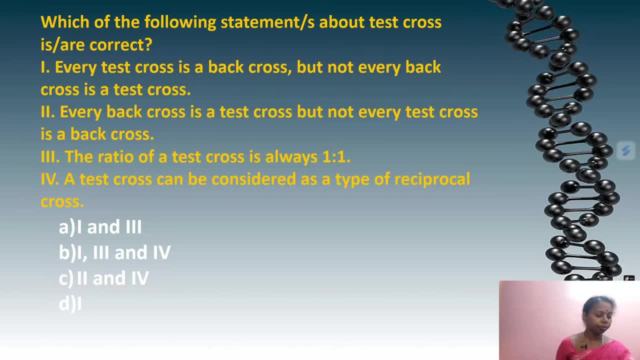 Jeevan Maalai Vanakkam Babadharini answered A. Jeevan answered A. So every test cross is a back cross, but not every back cross is a test cross is very correct, Because when you cross it with the recessive, it is a test cross. 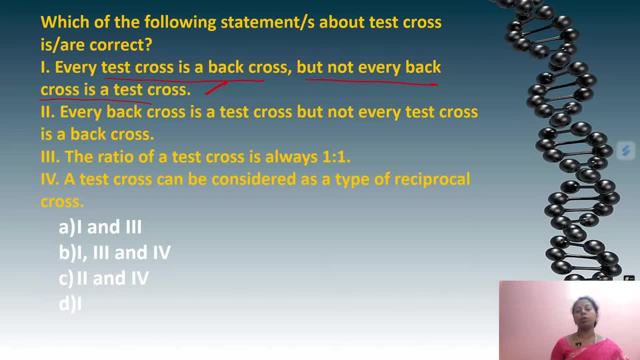 When heterozygous cross it with the dominant homozygous parent it is called out cross. So it is not test cross there. Very correct statement. And the ratio of test cross is 1 is to 1.. So every test cross is a back cross, but not every back cross is a test cross is very correct. 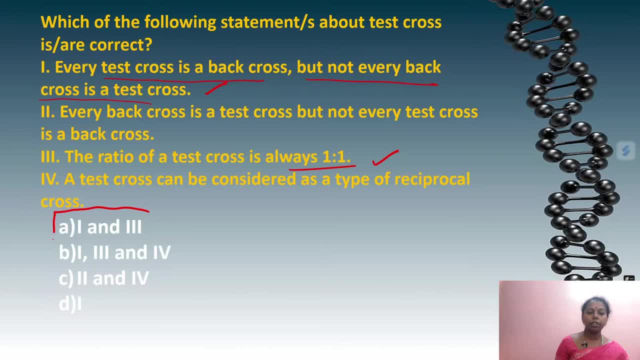 So the ratio is always 1 is to 1.. That is also correct. So 1 and 3 is the correct answer. Very good, Babadharini. Excellent answer by you. Very good, Keep it up. We are rocking today. 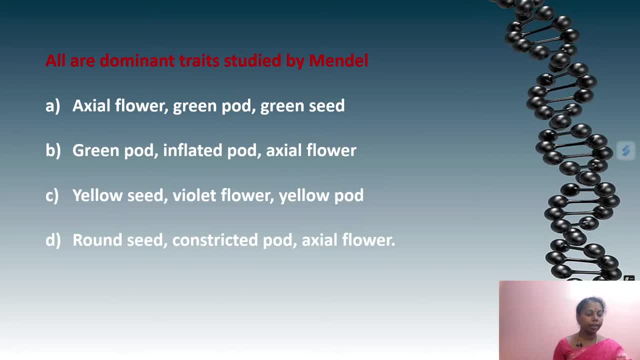 Fine. Next question: See, all are dominant traits studied by Mendel. Of course you know, Mendel studied some and contrasting, Dominant and recessive. So among this they are given some three characters which are dominant, Which among the three are: 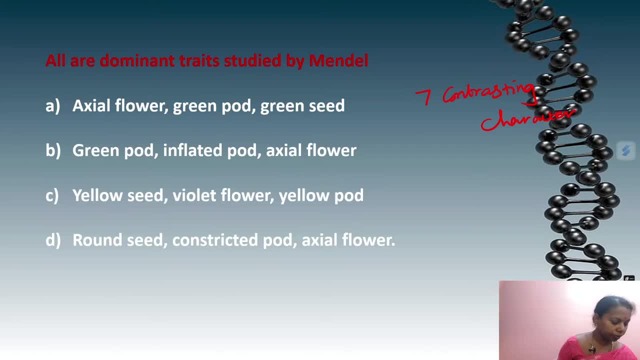 Only showing dominant is the question: What is back cross? and Yeah, thank you, Thank you. With all your support and love affection, we are reaching. We cross one year also. Yes, thank you, Sanjay, Yes, Dhani, coming to your, yes, Tamil New Year Day. 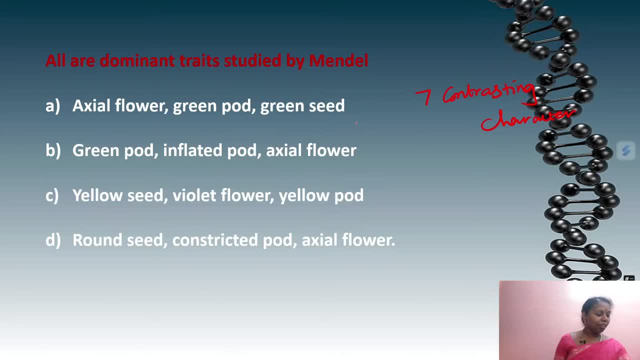 Happy Tamil New Year Day. So Dharani for you. yes, the love is always there with my children. yes, The love and support of my children is very helpful for me to reach this much. They are also motivating me. 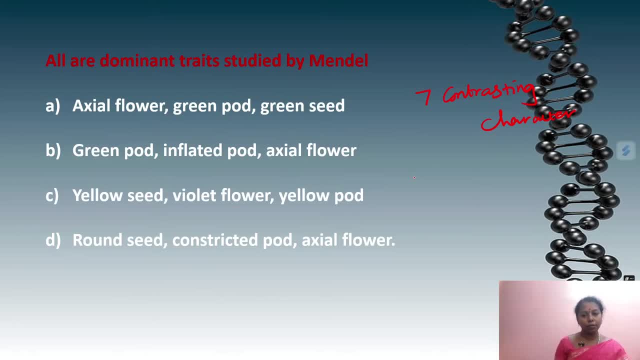 Okay, Yeah, Now we will clarify Dharani's doubt. Now what we do in test cross. Dharani, You are writing capital T, small t into small t, small t. That is recessive parent. If you cross the heterozygous parent, this is generally called test cross, isn't it? 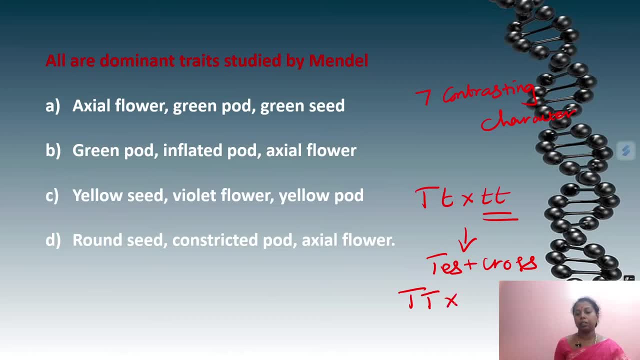 Yeah, This is also in back cross capital T, capital T into that is capital T. small t, That is heterozygous parent with a homozygous dominant. If we say this back cross as a men, we should also call it out cross. 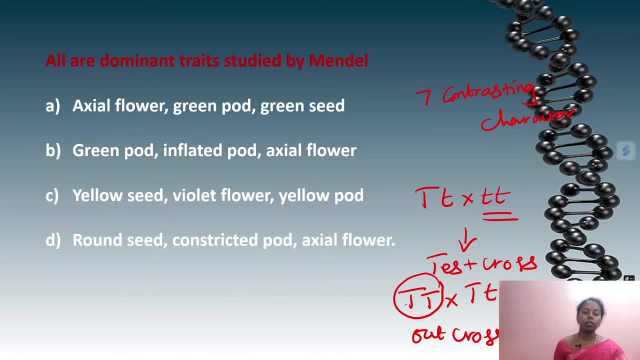 Okay, Yeah. So that is why all test cross are done as Yes, Okay, Yes, Yes, Okay, because there are some out crosses are also there. I hope I explained your doubt. so next week, if you have any topic, you can send it to me. 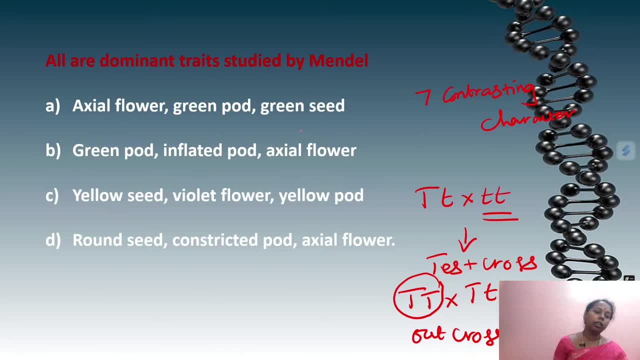 so that we can discuss it in the live itself. for every one of them it will be useful. so, all our dominant rights studied by Mendel. what is your answer? yes, Bhavadharani answered C. yellow pod. yellow pod is not dominant. yellow seed is dominant. yes, it is green pod. 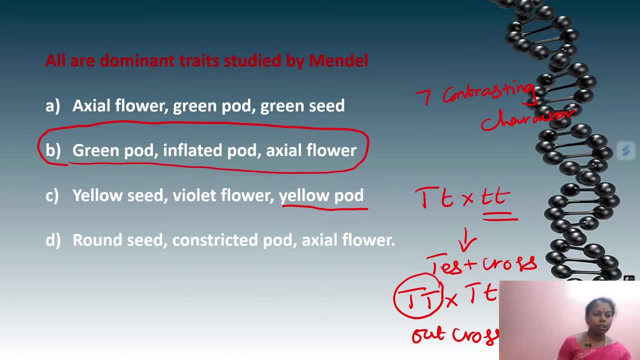 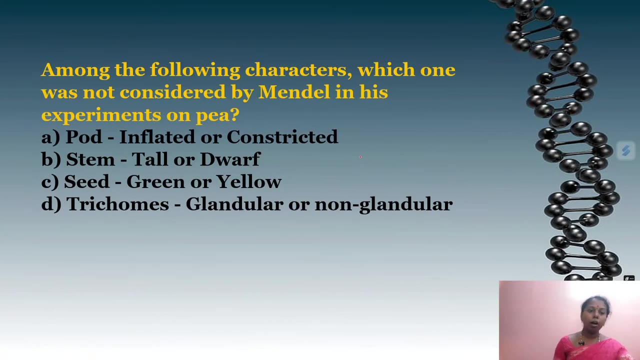 inflated pod and axial floor. all these three are dominant rights. yes, Lakshita and Dharani. yes, Sarunika, it is B. very correct answer, excellent answer by you all. very good, so let us proceed to the next question. among the following characters, which one was not considered: 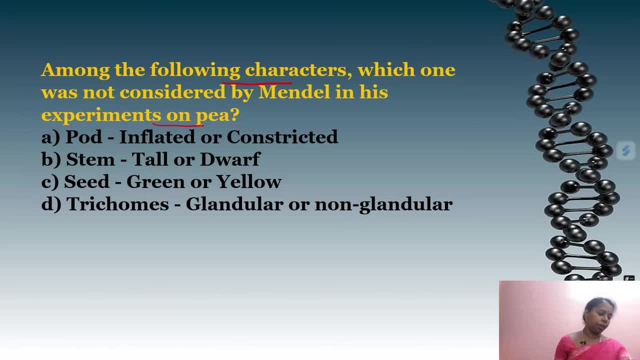 by Mendel in his experiments on P. yes, Sanjay, very good evening. yes, it is for the previous one, it was B. very correct answer. excellent answer, Sanjay, for that one. now for this question, which was not considered by the next question. yes, he considered pod, of course. 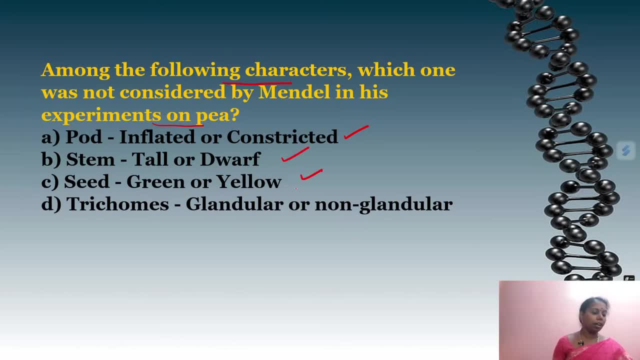 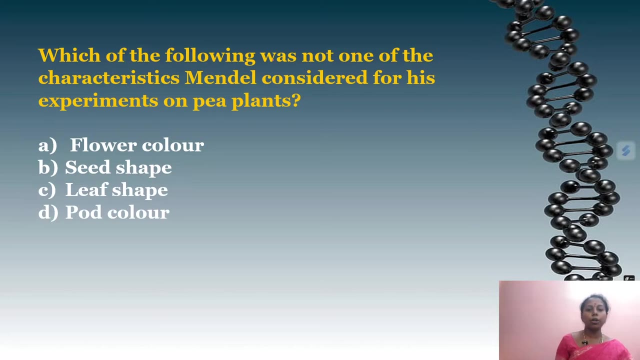 stem. taller dwarf considered seed green, yellow. of course he did not consider the trichome, which are glandular or non glandular, is the correct answer. very good children. yes, they are all rocking nice answers. which of the following was not one of the characteristics Mendel considered? 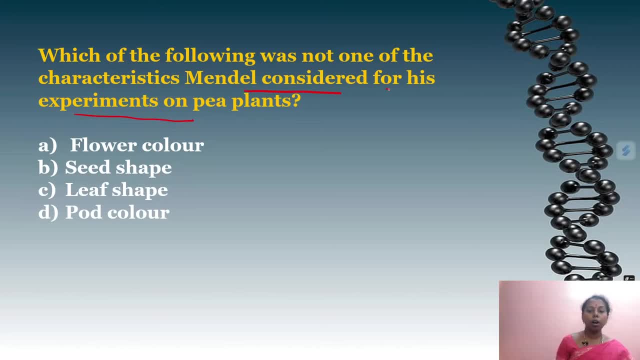 for his experiments on P plant. what is not considered by the Mendel? yes, he considered. yes, very good, excellent, you are rocking. yes, divan, very good, divan. now for this question, what he did not consider: we can use omitting option. so this color is violet and white. 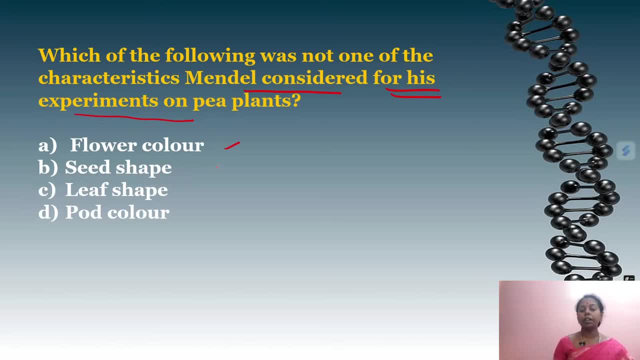 which he considered seed shaped, is inflated, which he considered is wrinkled or round inflated, or enens, which he considered in the pod. but leave avar yosike ve illa Illiya. So this is the correct answer, Excellent answer by many of you. 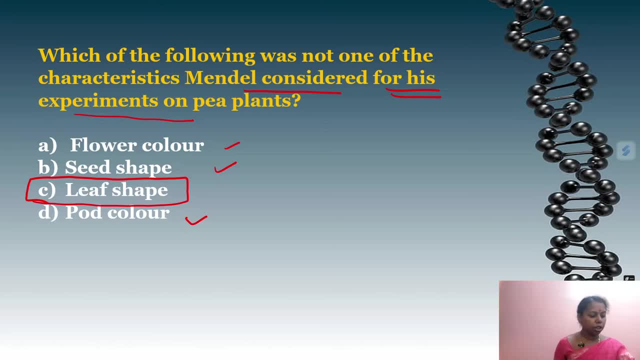 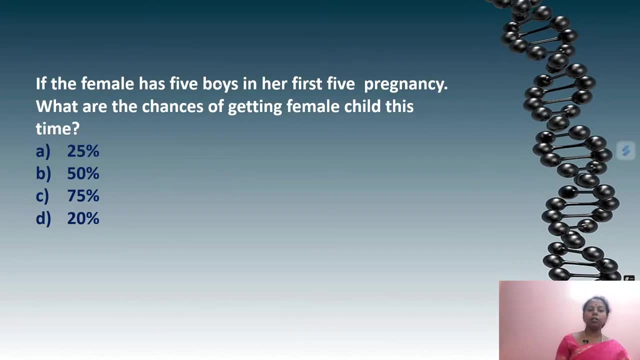 Yes, Sanjay, Lakshitha, Jeevan and Santosh. Yes, it is the correct answer. Very good all of you. Ippu inna. question paruna: If the female has 5 boys in her first 5 pregnancy, 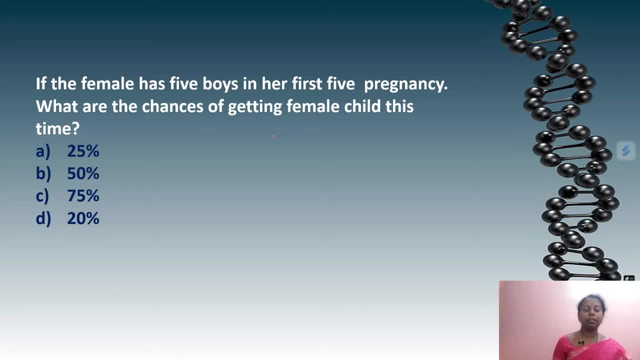 what are the chances of getting female child this time? Yes, Dhanashika, Very good, Good evening. Yes, it is D, Very good, You are rocking. Excellent answer by Dhanashika. So next question: If the female has 5 boys in the first, 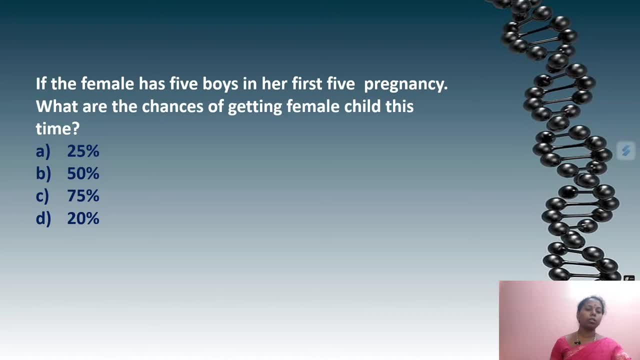 5, pregnancy next time. what is the probability of getting female child? Yes, it is B, Of course. I hope you all know this. So, XX crossing with X and Y, either we will get XX or XY. So 50 percentage of probability 1 by 2.. 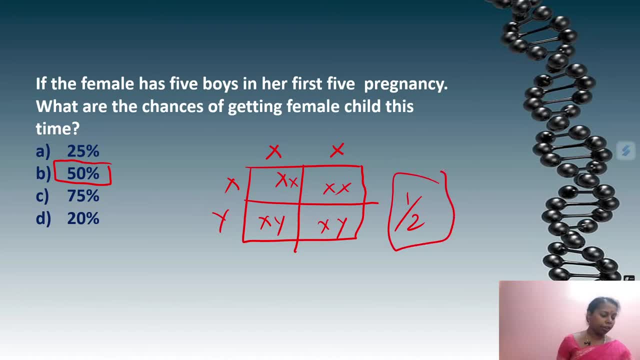 Either girl or boy. This is the answer. Okay, Very good. Excellent answer by Sanjay Santosh, Dharani, Bhavadharani, Lakshitha Dharanika and Dhanashika. Very good. 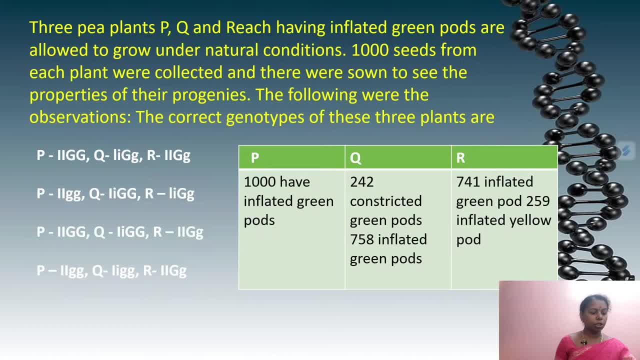 So next question- Literally, you have to think. Little lengthy question. also, Let me see who is answering first. So here we are having collection of 1000 seeds with the different characteristic feature. Okay, Yes, Jeevan, it was the correct. 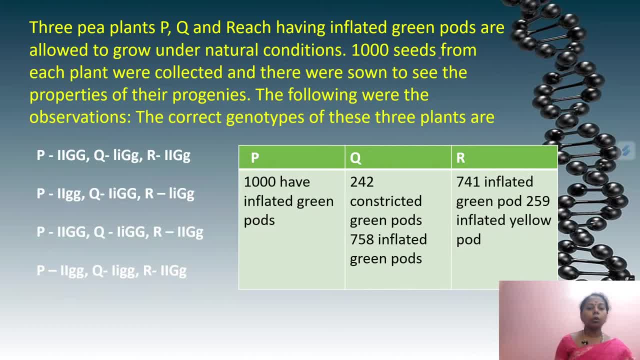 answer. Excellent answer by Jeevan. 1000 seeds from each plant were collected and they were shown to see the property of their progeny. The following are the observations. The correct genotype of these three plants are Dharanika. answered, That is. 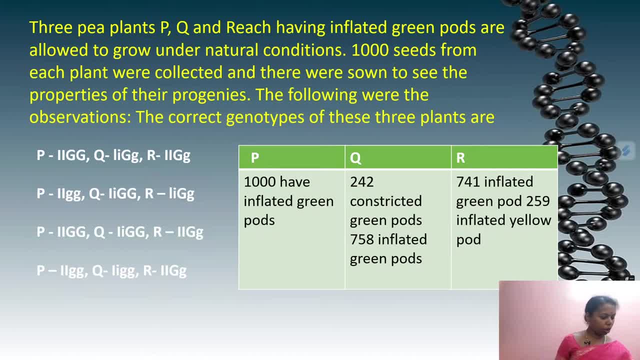 you are going with C option. Lakshitha, also C. C Dharani answered C Santosh answered C. Santosh answered C. Yes, it is C. If anybody is having doubt out, Let me solve the question. Yes, Sanjay, Let us see Thousand have inflated green pod. 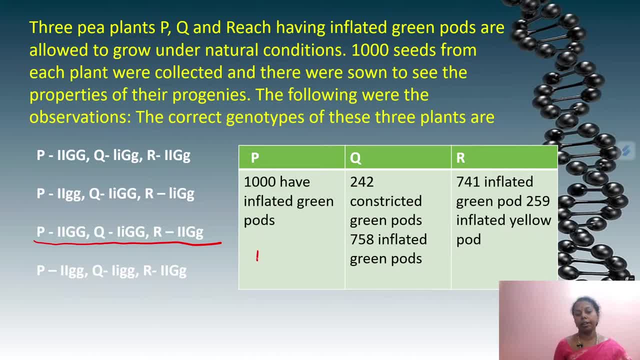 Inflated is a dominant character. Green pod is also dominant character. So we have to take capital I, capital I, capital G, capital G. So it satisfy P Q. let us see 242 constricted and 758 inflated. That means it is heterozygous Capital I, small i, But both are green pods. 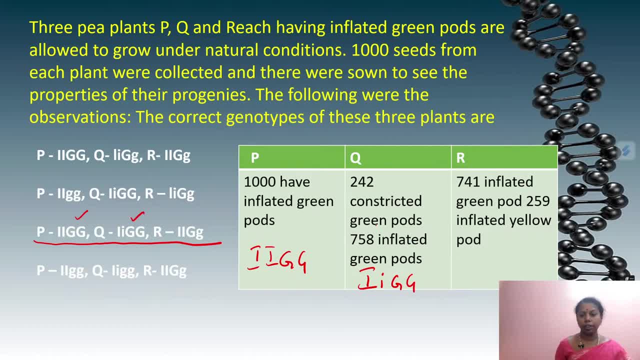 Capital G, capital G. So Q also is satisfied Here. if you see 741 inflated and 259 inflated, Both are capital I, capital I, But one is green pod, another one is yellow pod, capital G, small g. So this is the answer. The answer is in C. Yes, I explained the Bhavadharani. I hope. 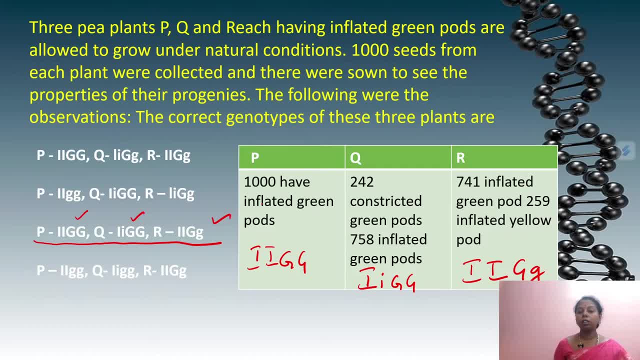 you understood. So just see: Thousand, all thousand. if inflated- this is the possibility- Inflated, we will take dominant character only. So capital I, capital I. Green pod is also dominant. So capital G, capital G. So where is that? 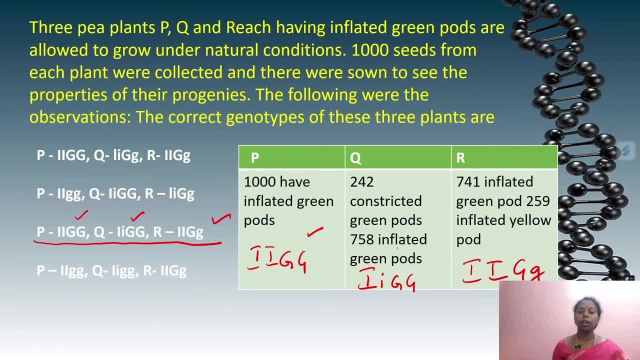 It is in P, Fine, Now in Q, constricted and inflated. So this is heterozygous condition. So capital I, small i, Is it in Q, Both are green pods, So it is dominant. So capital G. 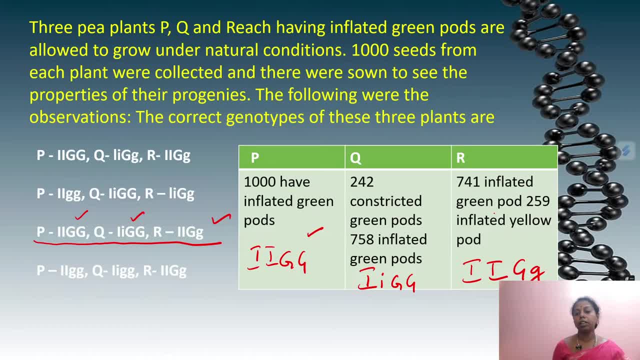 capital G Now, next is inflated. So capital I. capital I When we take green pod and yellow pod, it is heterozygous, So it is heterozygous condition. That is capital G, with the small g. 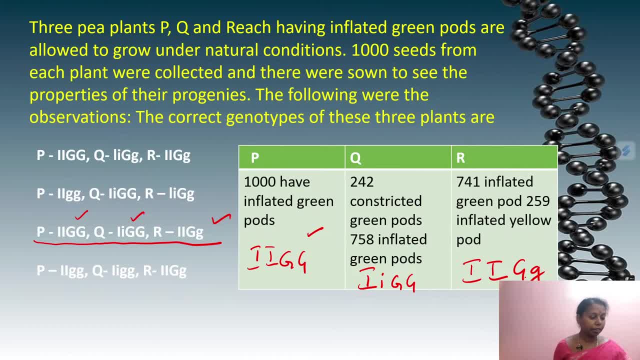 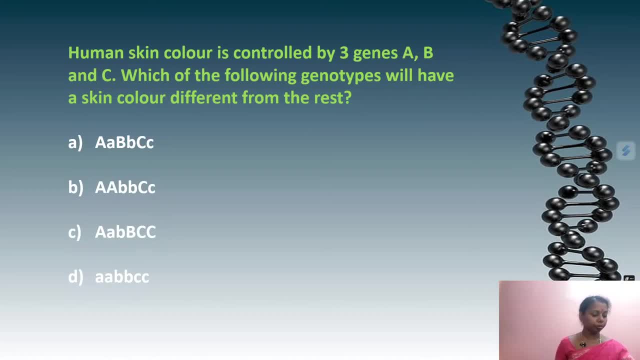 We take the condition this way. I hope you are clear now, Bhavadharani. Are you clear? Anybody needs still explanation. Yes, sir, Now we can see this question. Now we can see this question. Now we can see this question. 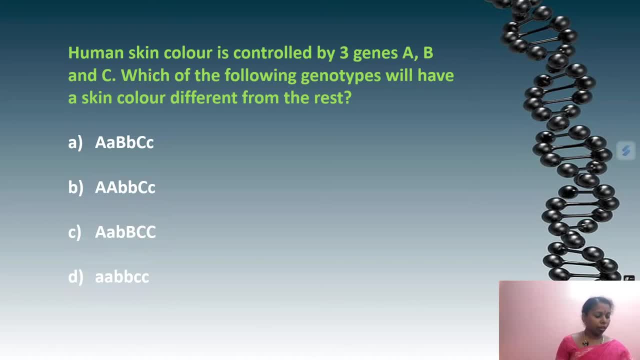 yeah, thank you. yes, vivekananda, very good evening. human skin color is controlled by three genes: a, b and c. which of the following genotypes will have a skin color different from the rest? so it gives a black color. so melanin will be more and black will be more. 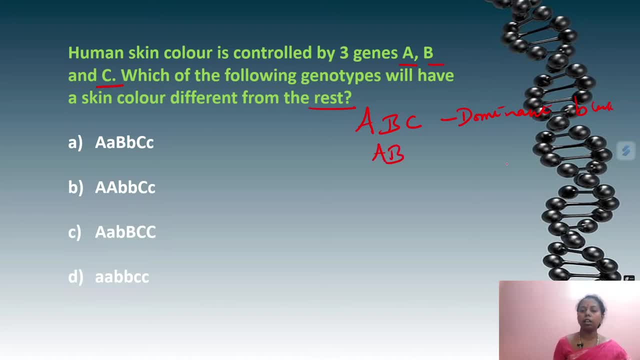 if we have two dominants, then the coloration will be less. if we have only one dominant, then it will be less. if there is no dominant, then it will be less. that means they are albinos. so in the answer given here, where they are different, of course d is the correct answer. 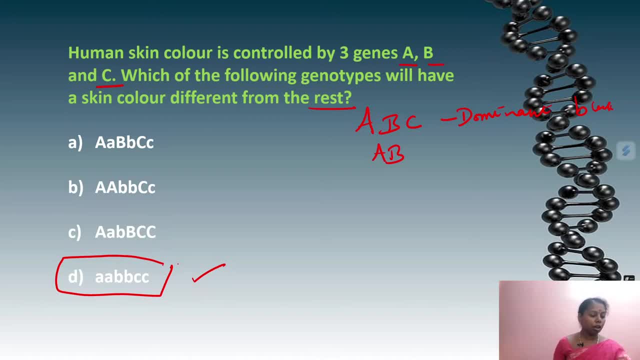 where they do not have any melanin pigment. so they are completely albinos. yes, santosh, excellent answer by santosh. yes, santosh, excellent answer by santosh. and bhavadharani: yes, very well done, children, all of you. now next question, a little tricky question. 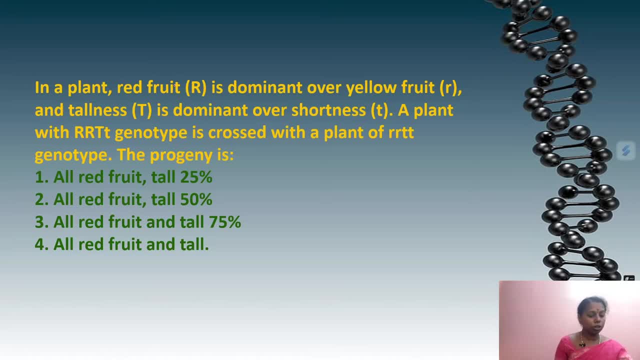 you have thought about it a little and answered it: the tall in a plant, red fruit is dominant or dominant over yellow fruit. so whether red fruit is capital or capital yellow, we take as small or smaller. and tallness, as always, we take as capital T, shortness as small T. 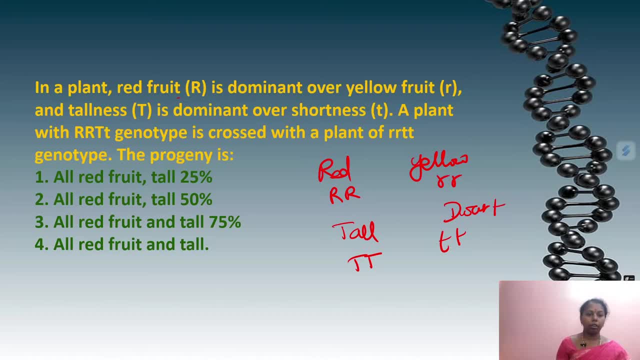 and shortness as small T and shortness as small T. that is love. then, capital R, capital R, capital T, small T genotype is crossed with smaller, smaller, small T, small T genotype. what is the purpose of this is what you have to ask before I complete. yes, very good, dharnika, excellent answer by you. 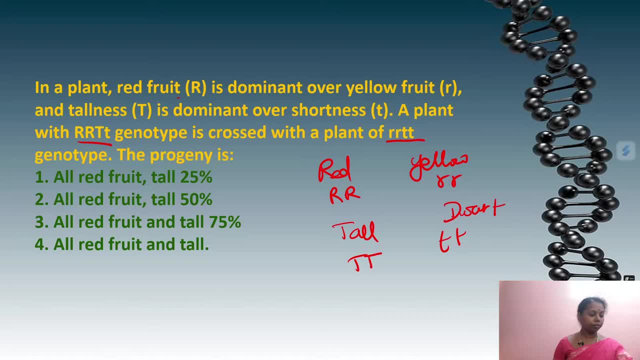 we will see, wait and see. others are how they are answering. yes, very good, dharnika. excellent answer by you. we will see, wait and see. others are how they are answering. Yes, Lakshitha, also go with Dharanika's answer. Dharani answered. 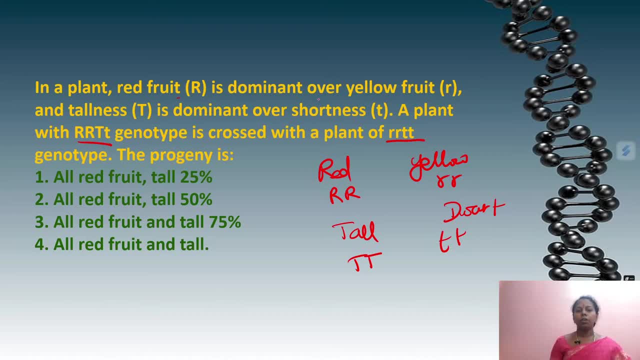 See those who are listening or observing the class. you can even answer all time. It won't be correct. Even when we make mistake. we will learn children, This grouping and discussing the answer. it will reduce our stress. So please answer children. 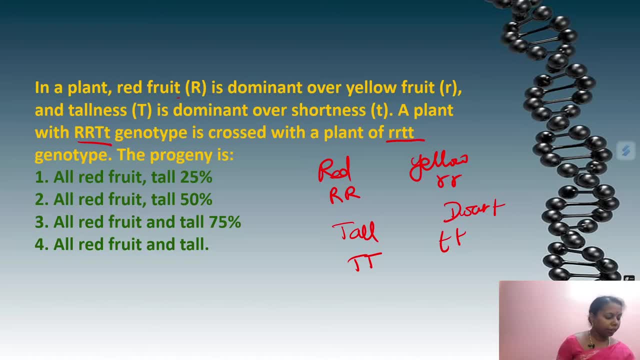 Yes, and Santosh answered too: Yes, it is a test cross, Very correct. See, we can't say heterozygous, Only tallness is heterozygous Here, when you put capital R, capital R, small r, small r. 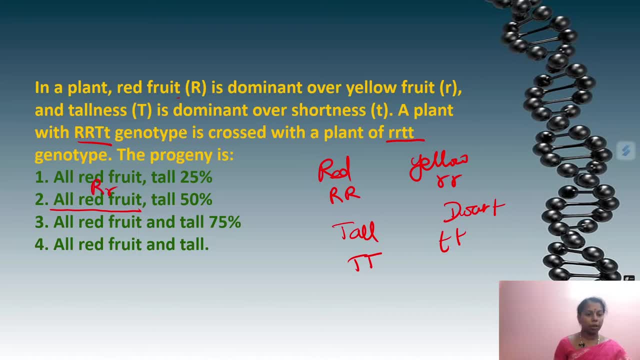 all red fruit will come. That means capital R, small r, And when you put capital T, small T, small T, small T, tall and dwarf will be 50-50.. So here he gave the answer: Tall is 50%. 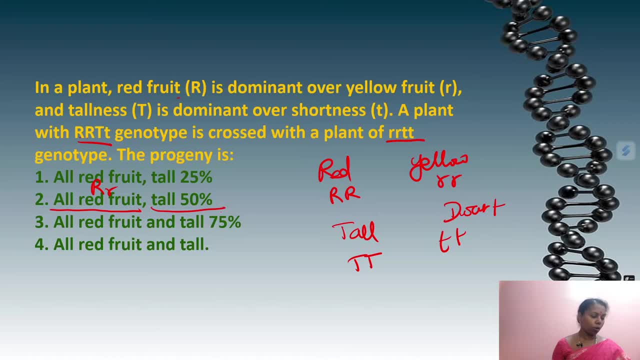 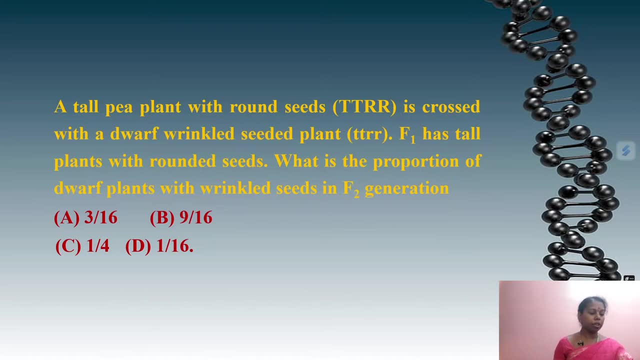 So that is the correct answer. Okay, excellent children. Now next question, We are proceeding. It was very correct answer. Excellent answer by you all. A tall pea plant. In the question we see tall pea plant has round seed. 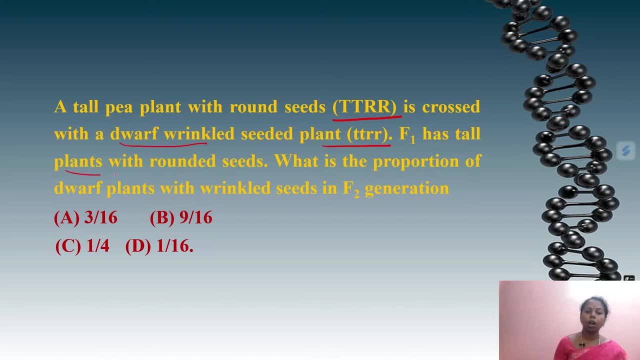 Dwarf wrinkled seeded plants have round seed. F1 has all tall plants with round seeds. What is the proportion of dwarf plant with wrinkled seed in F2 generation? That is the question. So when weIK супnot ask these questions with attention? 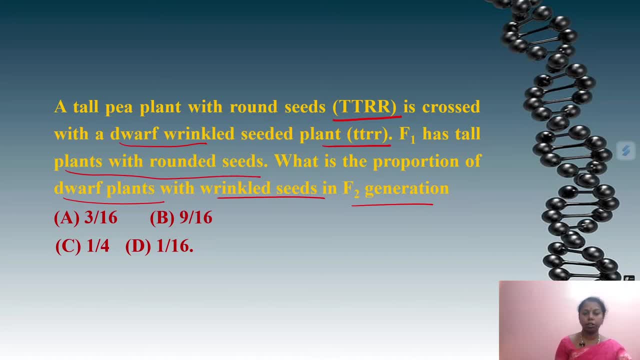 our concentration and focus should not get derat in the question. if i miss a word may cause lots possibilities for us to make mistake, Am I right? So don't do like that. I will share the tale I know here One timeーネ鳶. 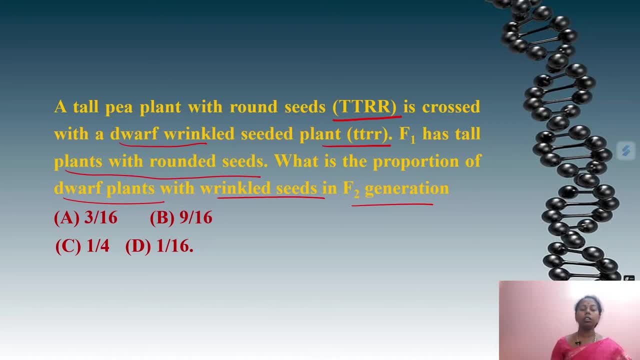 Dronacharya came and went and learnt dhronacharya's story. He was asking everyone to focus on one sparrow. Everyone was focusing on the sparrow and the parrot. He asked everyone what they were looking at. Dharampar said I could see the branch of the tree, the leaf, the bird's leg. 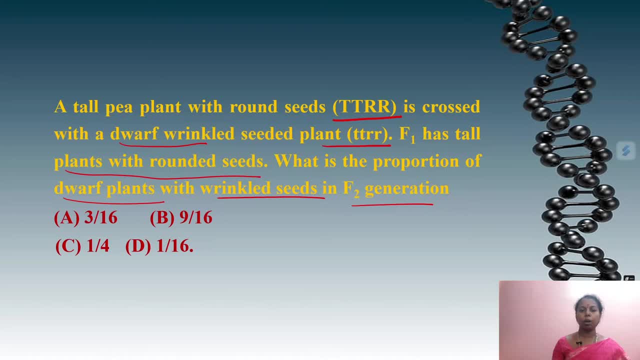 Dharampar said I could see the branch of the tree, the leaf, the bird's leg. Dharampar said I could see the branch of the tree, the leaf, the bird's leg. Everyone was focusing on the arrow. 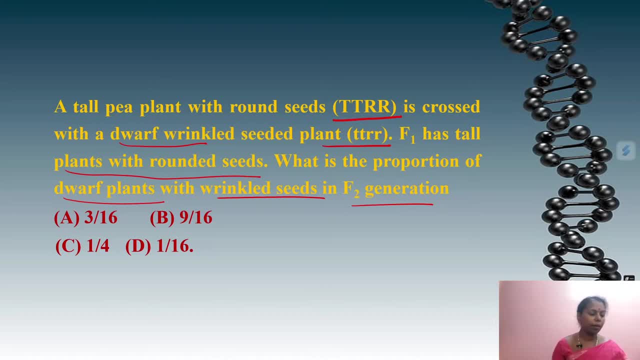 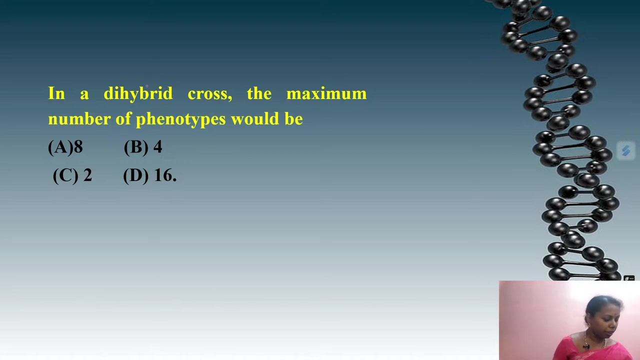 We can concentrate on the arrow and not make mistakes. I hope everyone was focused on the arrow. 1 power 16 is the correct answer. 1 power 16 is the correct answer. Excellent, all of you children, Yes, Babadharani Nandika and Lakshitha Dharani Santosh. Yes, it is 1 power 16.. In a dihybrid cross, the maximum number of phenotype would be. So how many number of phenotype is possible in a dihybrid cross? Yes, it is 4.. Very correct, As you know, 9 is 2,, 3 is 2, 3 is 2, 1.. 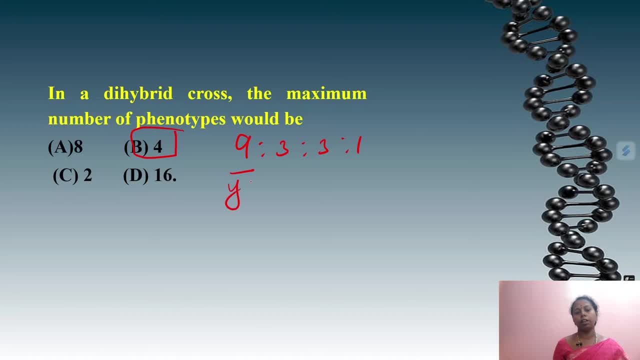 So 9 is yellow and round. This is yellow and wrinkled, Green and round, Green and wrinkled. So did we get 4 phenotype or not? So this is the correct answer. excellent answer by you all, children, Yes. next question is: we are making the genetic map. 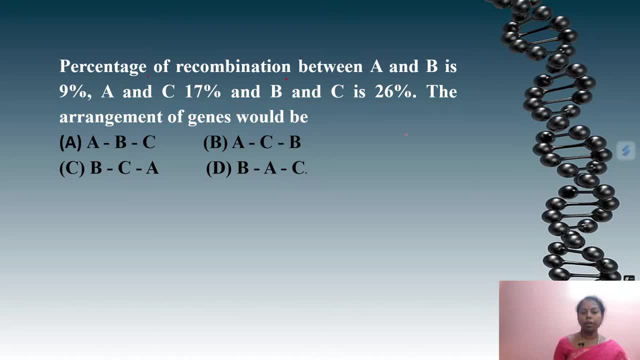 Percentage of recombination between A and B. how much is given A and B? is equal to 9%. How much is given to A and C? It is around 17%. So B and C- how much is given? It is around 26%. 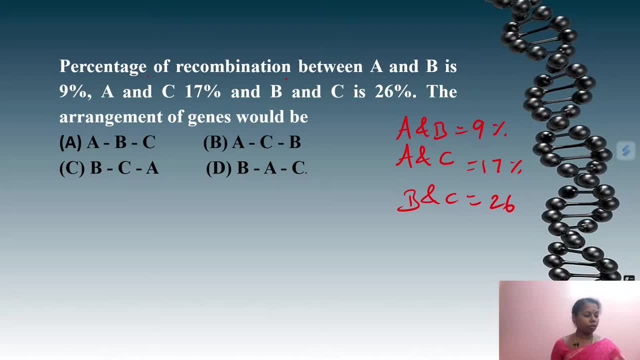 How would be the arrangement of genes? Ask such questions, So you have to find the answer now. BAC DN: Kodre Ganga Tarunika, We will see. Yes, Lakshitha, Yes, it is correct actually. 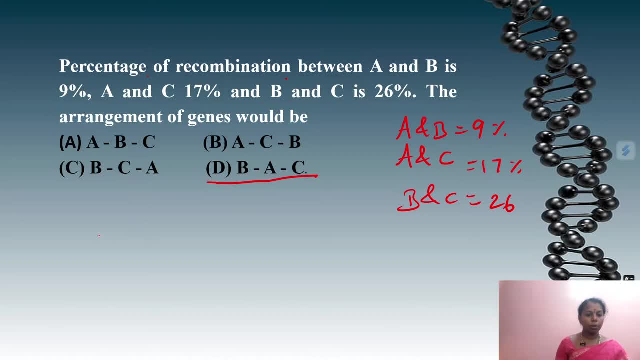 Excellent answer. It is BAC Bhavadharani. Yes, So we should always take B and C as 26.. So if we take B and C, what is there between A and B, 9.. So if we take 9 from B to A, the rest of the 17 comes to A and C. 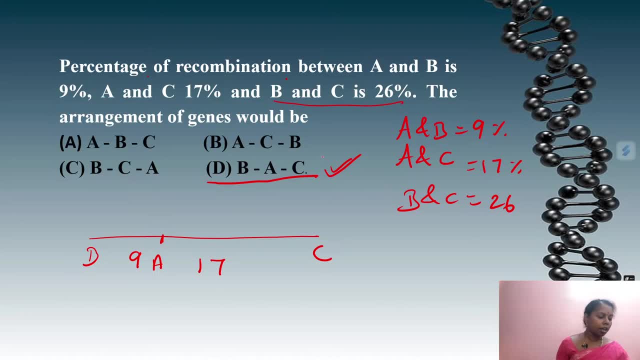 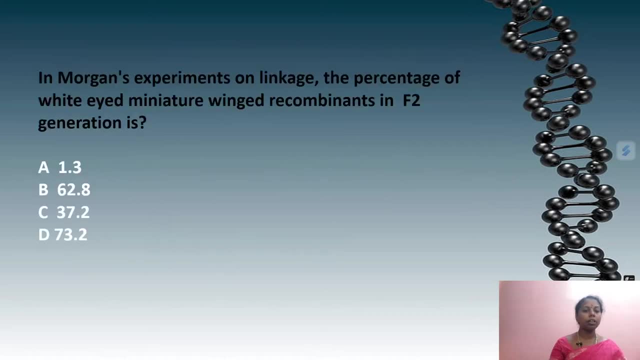 Yes, So totally it is 26.. The answer is very correct. Excellent answer by Dharani and Bhavadharani, Lakshitha Tarunika: excellent, Very good, Excellent. They are all rocking. Now next question. 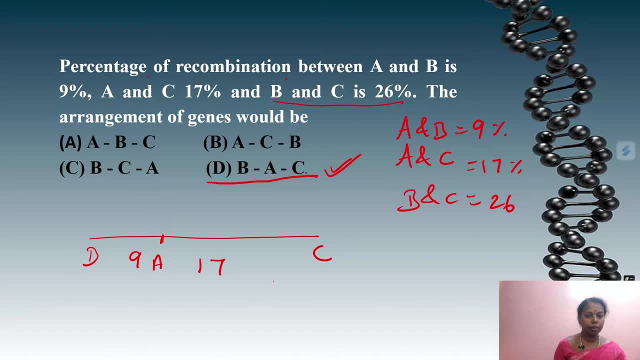 Yes, Santosh. Now in this question we should always take the big number, So B and C is 26.. We did not give that number in the other questions, So what we did was we took B and C. 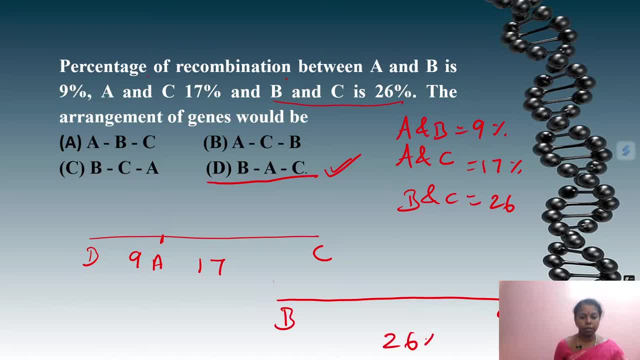 Between B and C. we have 26 percentage. So between A and B, what is there between 9?? So this is A, So this is 9.. So between A and C, what is there between A and B? 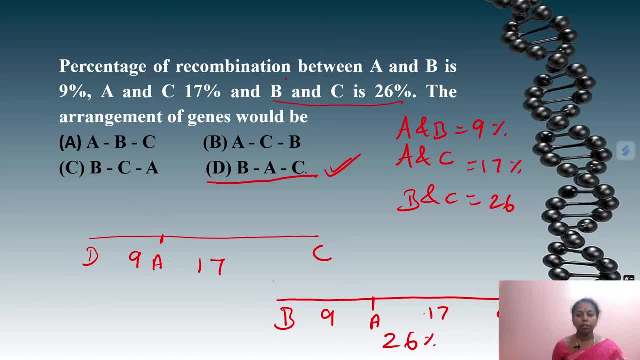 17.. So if you add these two you will get 26.. So B and C is 26.. So the arrangement is B A C. That is the answer. I hope you understood, Santosh. Are you clear now? 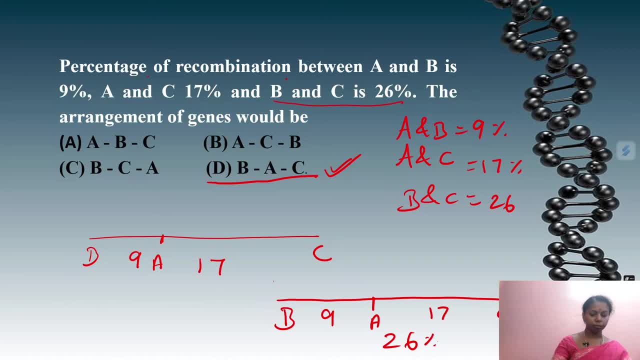 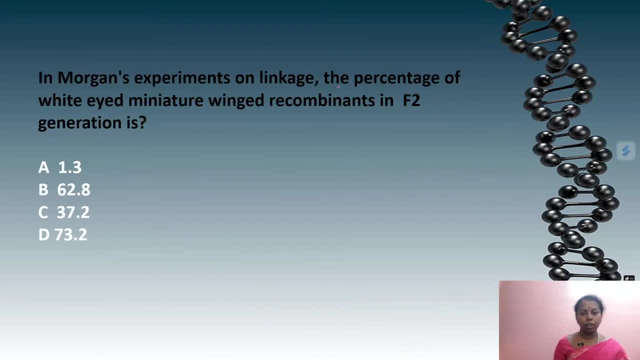 Shall we proceed to the next question? in Morgan's experiment on linkage, the percentage of white eye miniature winged recombinant F2 generation. so winged eye miniature recombinants, white eye miniature in recombinant. it's a NCRT line and the linkage 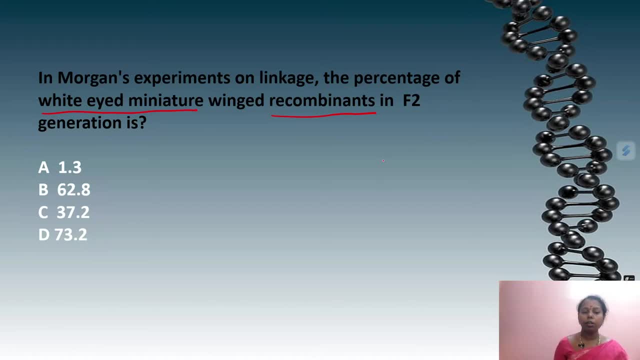 there is a diagram, chromosome diagram. there recombinant value is given. that is the answer. yes, Santosh, thank you. so now answer for this question. so what is the recombinant percentage in red? yes, yes, Arunika answered, it is 37.2. 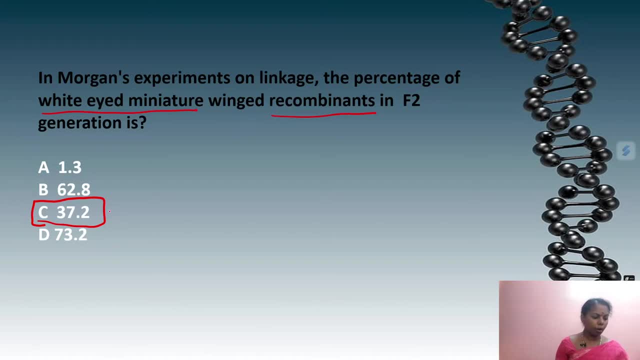 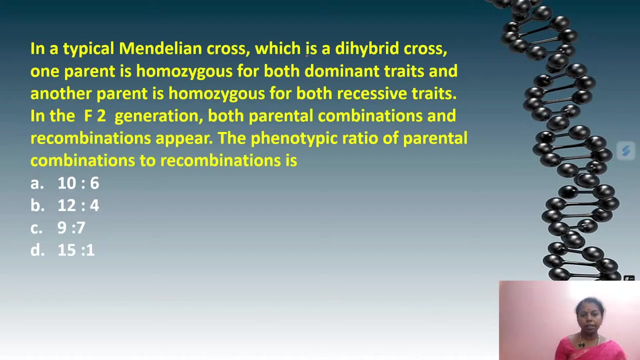 NCRT line of course 37.2 is recombinant, recombinant, very correct. excellent answer by Lakshita and Tarunika: yes, Darini also and Santosh, yes, very good. now next question: NNPOP in a typical Mendelian cross. 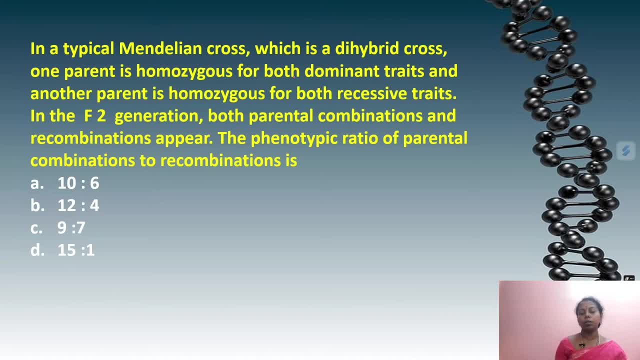 which is a diablet cross. one parent is homozygous for both dominant trait and another parent is homozygous for both recessive trait. in the F2 generation both parental combination and recombination appear. the genotypic ratio of parental combination with recombination is: 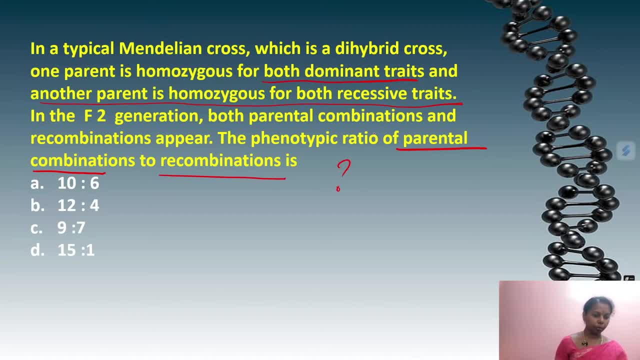 how much? Yes, so if you take the dihybrid cross, 9 is to 3, is to 3, is to 1, this 9 is parental combination- yellow and brown, green and wrinkle is also parental combination, which is 10, and these: 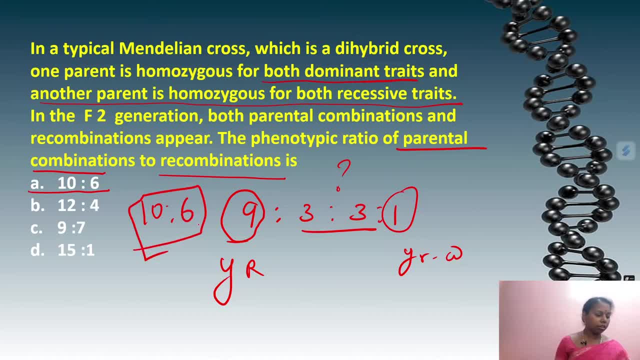 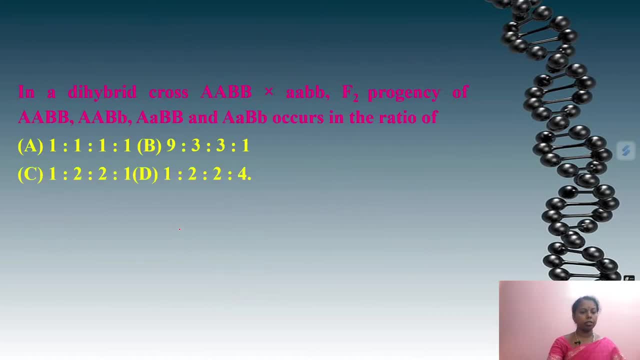 2 are recombinant, so 10 is to 6, this parent versus recombination. very correct answer by Lakshita and Dharani. yes, very correct answer. excellent all of you. Now this question: capital A, capital A, capital B, capital V is crossed with small, a small. 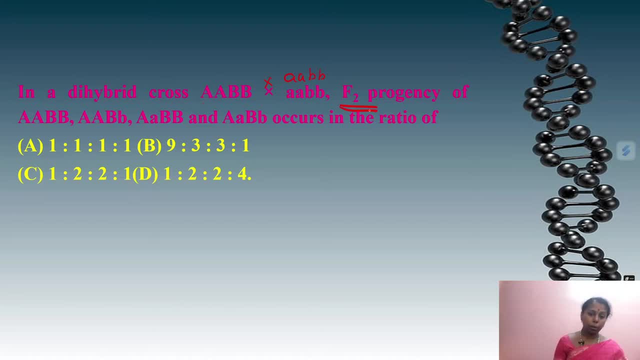 a small b, small b F2 progeny. please remember F2 progeny. what is the probability of getting these offspring? Yes, very good. yes, yes, it is C. let us see so easy way of crossing capital A, capital A, into. 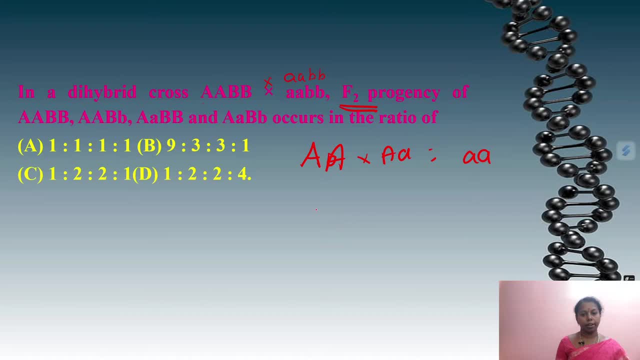 capital A, small a is to small a, small a when you cross with capital B, capital B, capital B, small b and small b, small b. first one: everything dominant, this is also 1, this is also 1, so 1 is correct now. second one: capital A, capital A. 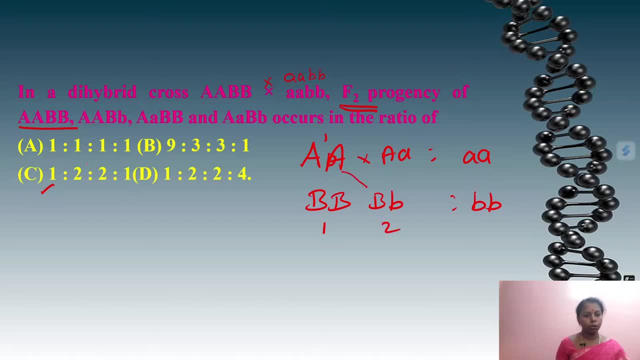 capital B- small b. this and this. this is 2: 1 into 2, 2 correct. now this is capital A- small a and capital B- capital B, 2 into 1, of course, 2 very correct. and last one, capital A. capital A is 2. 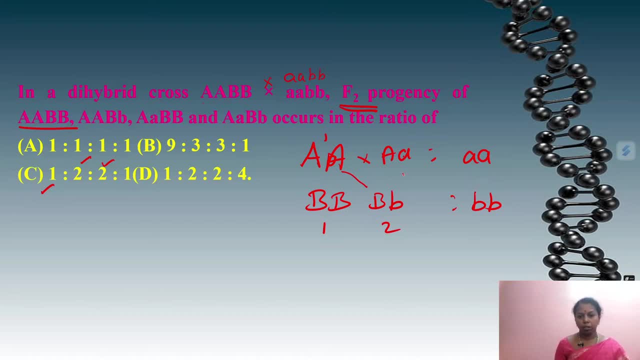 capital B, small b. That means 2 into 2, 4.. So the answer will be in D option. Yes, sir, So that is why we missed our focus here. So the last one, if you see, both are 2.. 2 into 2. 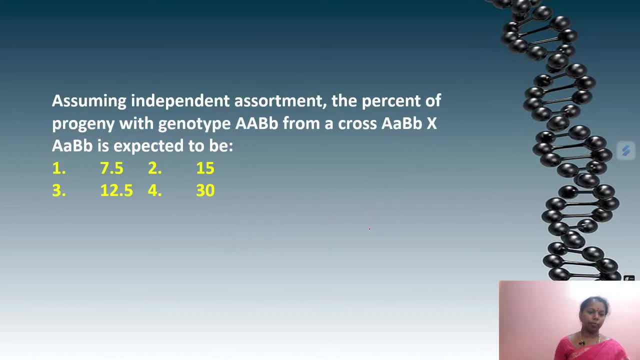 it will become 4.. Am I correct? children? Yes. Now next question: Assuming independent assortment, the percent of progeny with the genotype capital A, capital A, capital B, small v from across of capital A- small a, capital B- small v. 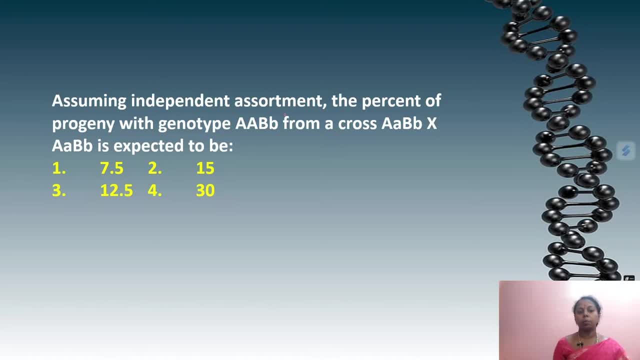 capital A small a. capital B small v is expected to be. So they are asking this genotype ratio percentage. So those who are observing the class, please feel free. I am your teacher, You can answer. even if it is wrong, We will. 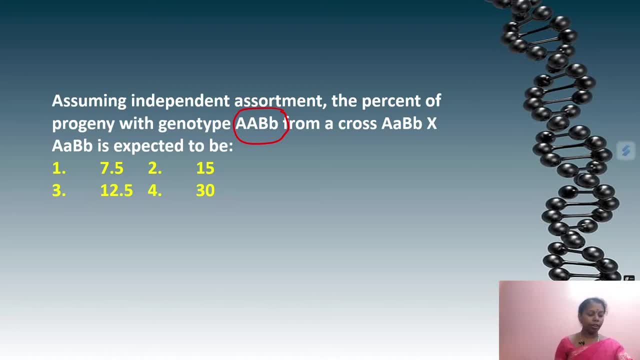 be learning. It is not that delay. Any explanation is needed. I will tell you. Tarunika answered C. Nandika answered C. Tarunika answered C. Yes, it is C. Very correct answer. Excellent answer, children. 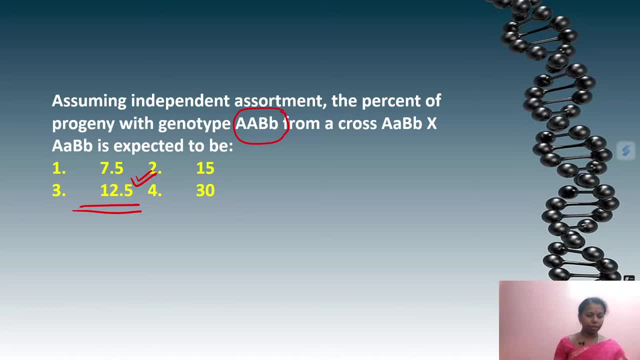 All of you, It is C only If you do the same cross capital A small a, 2, capital B small v, also 2. 2 into 2, 4. 4 bar 16.. Okay, So whatever you will get. 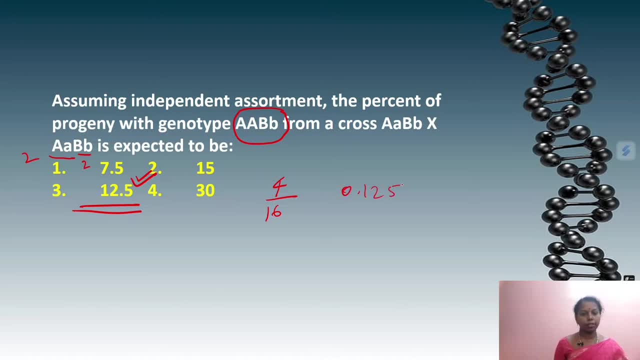 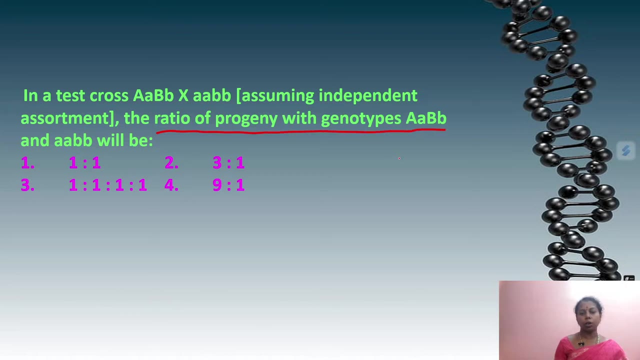 is something like 0.125. as it is 100%, it will become 12.5, is the answer. Okay, So it is C is the correct answer. Very good, Now what is the ratio of progeny when we cross Capital? 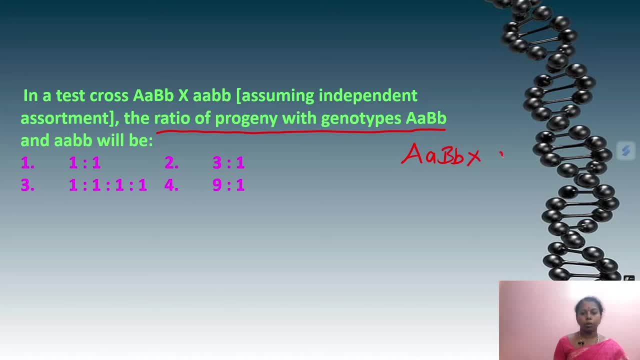 A small a capital B small b into small a small a small b small v is the question. So if you practice these sort of question it will be more interesting. It is easy also to pitch them up. You don't want to remember anything. 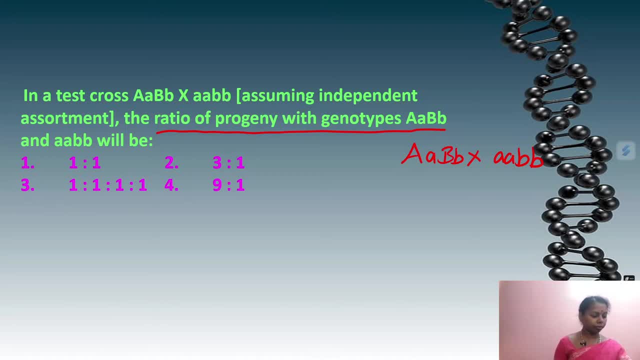 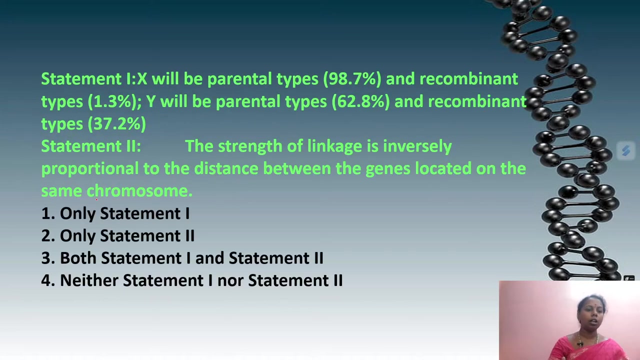 Just you can work out an answer. 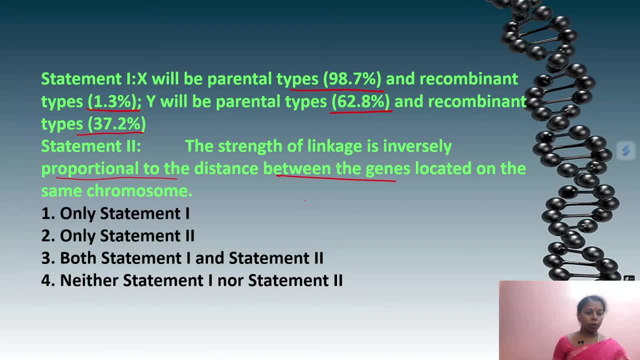 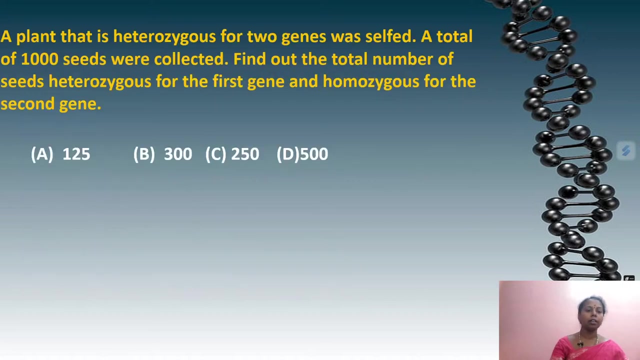 Heterozygous for the first gene and homozygous for the second gene. I hope you understood. 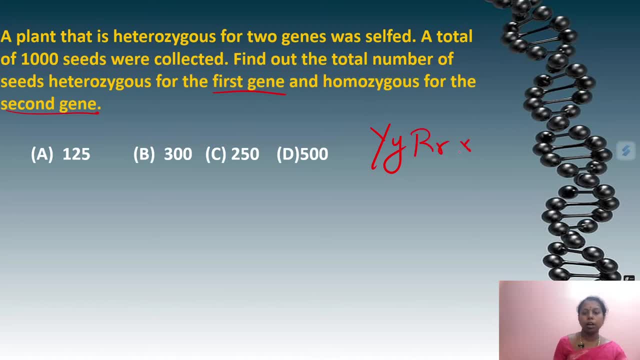 They are crossing YyR into YyR. They are asking: first gene should be homozygous and second gene should be sorry, first gene is heterozygous. homozygous for the second. See, there is a king, okay. 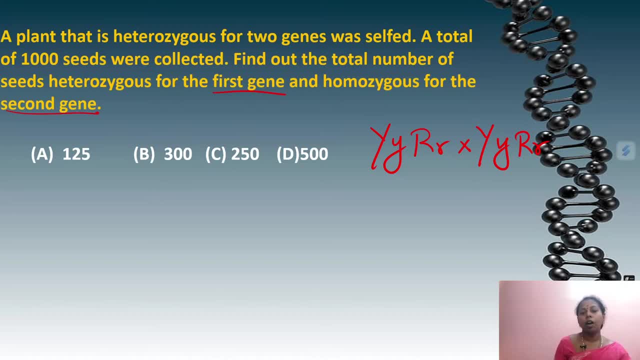 Yeah, and the king has three sons. He wants to find out who is the most talented among those three sons, because he wanted to give his kingdom to rule To one of his sons. So to find out who is the most talented among those three sons. 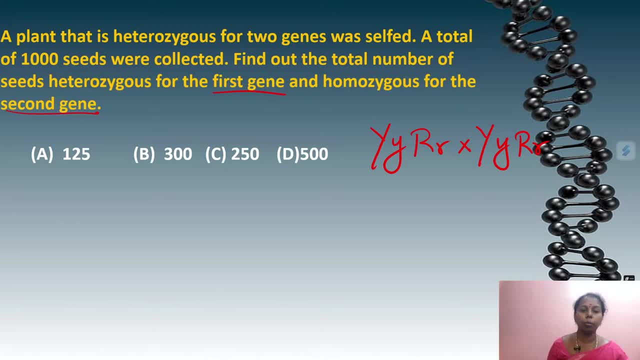 he wants to bring a mule who lives in a very deep forest. So they are going, Okay. when three of them are going, the first thing a boy hears is a laughing sound. There is a good smell, a lavender smell. 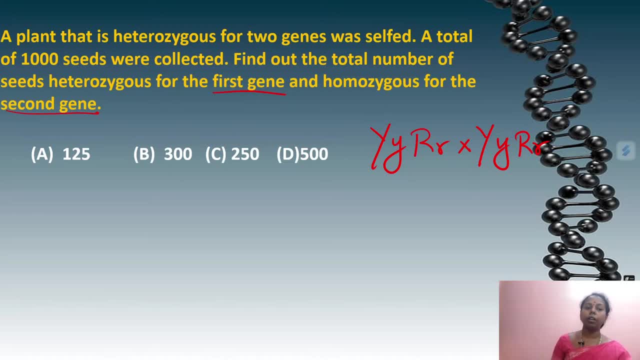 What does he do? He deviates to the other side and goes away. The second, the two of them are going. they are proceeding. So when the second boy goes, he hears some sound like a fighting sound. What does he do? 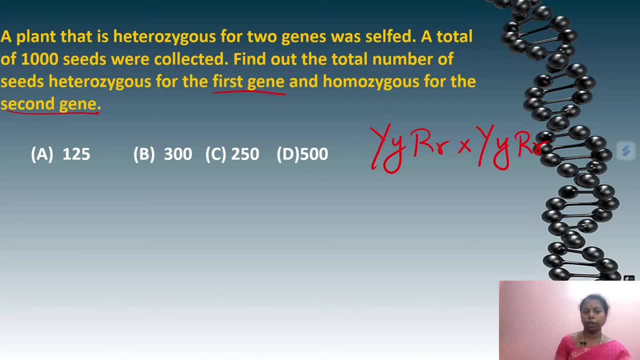 He says, let's hear what sound this is. and he deviates to the other side and goes. So what does the third boy who is going do? He is going straight in that way. When he goes in that way, at the end he gets his Achyuthat goal. 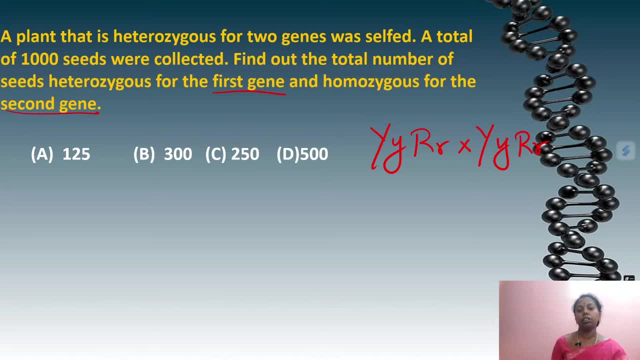 his medicine- his mule, By the way- he is going in that direction and then he goes up towards the front, and then he goes out and gets up, Then he goes back in the same direction and his camera goes in the opposite direction. 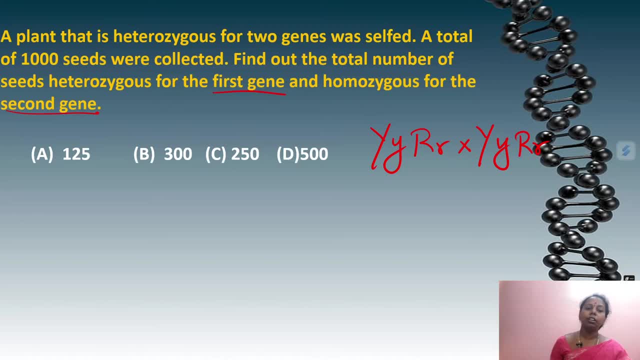 and he goes back in the same direction. This is a very interesting opportunity, But we can see, if the third boy goes to the front, he will not be able to go back to the front, Yes, And he will just go back and come out of the front. 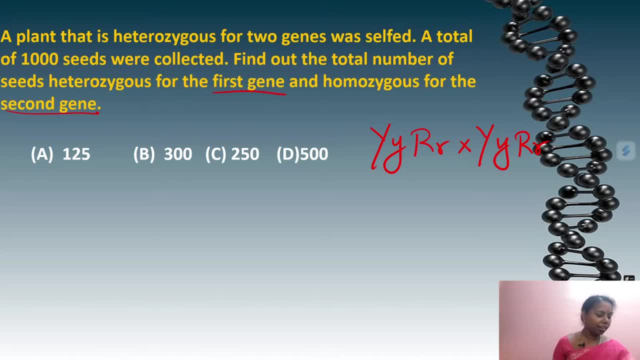 This is an interesting opportunity for us to find out how he is going now. So what do we know about him and what he will do after that? We will see that later, If you have not seen it before. when you work out, first gene of heterozygous is capital Y- small y, and second gene, homozygous, is capital R, capital R or capital Y, small y, small r, small r. 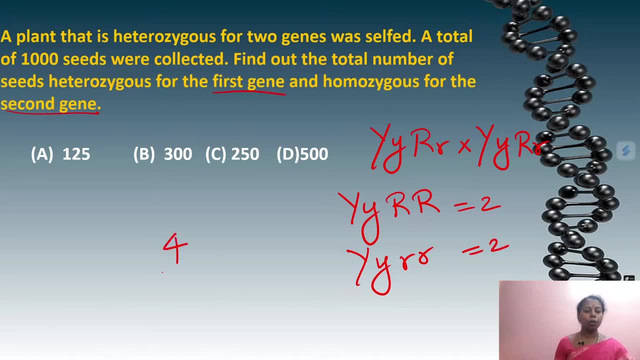 So totally, 4 bar 16 into 1000, what will be the answer? 125.. So we will get 125 seeds of this criteria, So A will be the answer. I hope you all understood, Anyway. so you were all answering. very good, This is a tricky question I can understand. Now let's see this question. 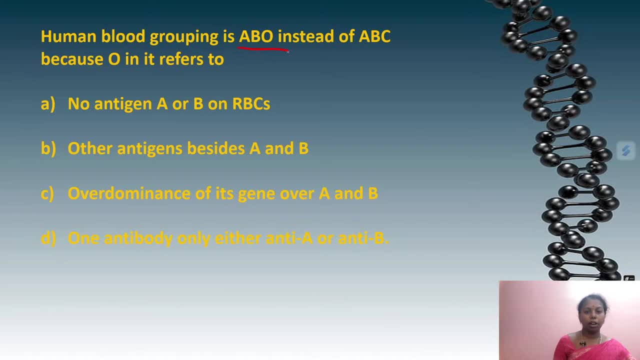 Our human blood group is In our blood group. A, B, O. are there right? Why C? Why they mention it as O? Why not? it is C, Yes, Yes, very good, There is no antigen. Yes, Dharanika and Lakshitha. 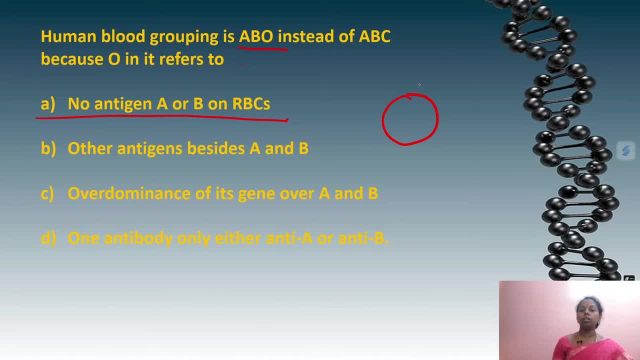 So antigen is not on the surface. This is what Western countries call 0. So we call it O blood group. When there is antigen, we call it A, B, Yes, very good. Dharani, Daniel and Nandika. 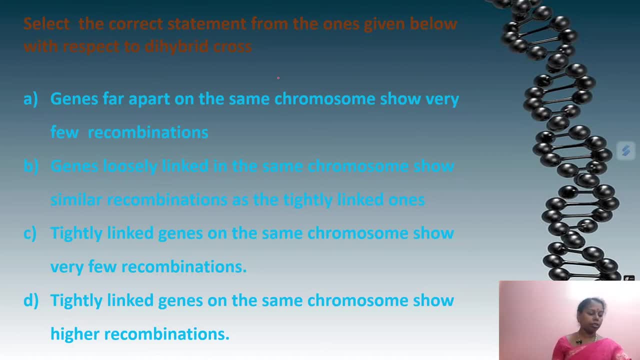 Excellent answer by all of you. Now, this antigen In this statement, which is the correct statement, we are going to find. Genes far apart on the same chromosome show very few recombination. Genes loosely linked in the same chromosome show similar recombination. 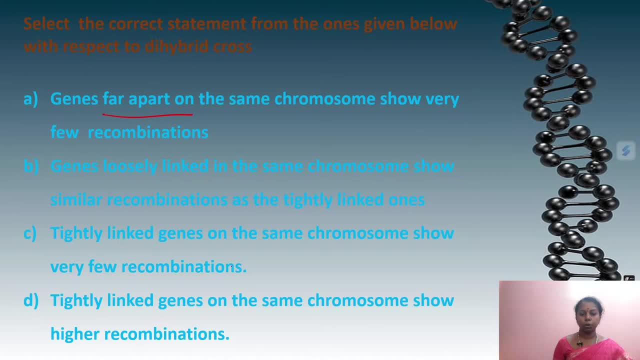 Tightly linked genes on the same chromosome show very few recombination. Tightly linked genes on the same chromosome show higher recombination. What is the correct answer? Yes, Santosh, you are rocking. Very good answer For the previous one. Now for this question. 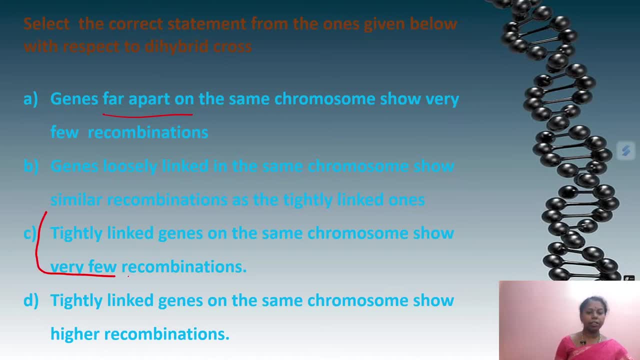 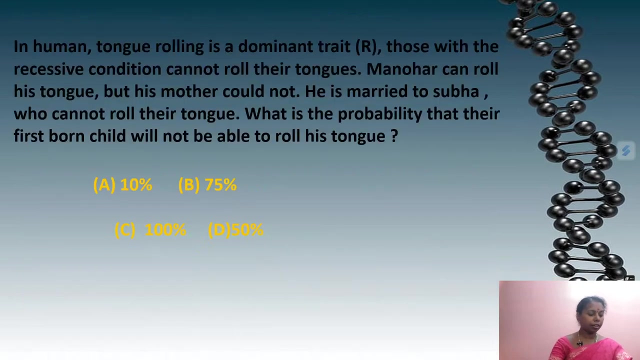 Yes, Daniel. Excellent answer, Daniel. Tightly linked genes on the same chromosome show very few recombination. Recombination will be very less for those tightly linked genes. Very correct answer. Yes, Santosh and Dharini. Very correct answer. Excellent, all of you You are rocking. Yes, Nandika. 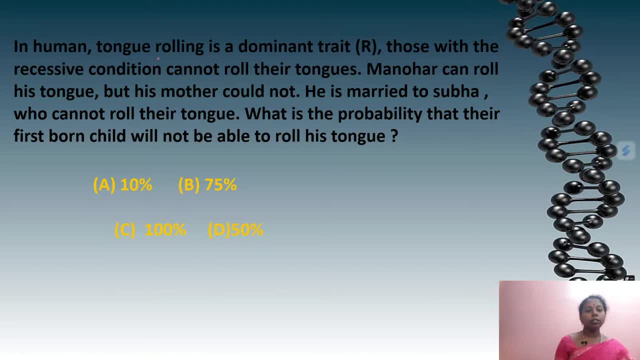 Now let's see this story. Human tongue rolling is dominant, right, So some of you can roll your tongue, which is dominant. Those who are with recessive, they cannot roll their tongue. Now, in this story, Manohar can't roll his tongue. 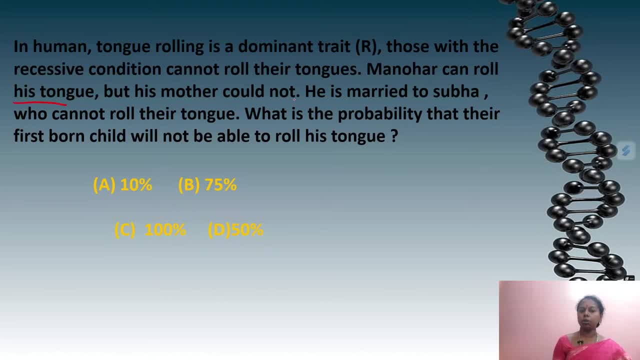 Manohar can roll his tongue, So he can roll, But his mother could not. He married to Subha, who cannot roll her tongue. So what is the probability of their first born child will not be able to roll their tongue? Yes, Arunika already answered. She answered for 50%. Let us wait and see what others are answering. 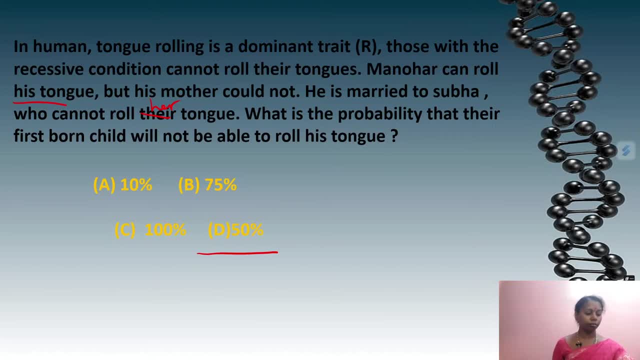 So any doubtful question, any doubtful topic, you can send it to me through comment or WhatsApp, which will be discussed in the next live class. It will be more useful to you, children. Please feel free and send your doubts with reference to NEET syllabus. 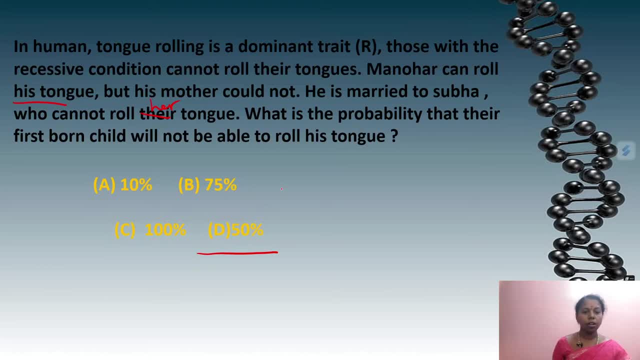 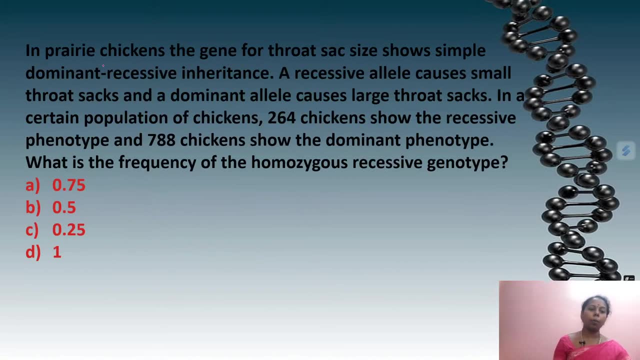 Yes, it is D, Very correct, Excellent. So half of the children can roll their tongue and he will be atrocious, I guess. No, Manohar. fine Now priori chickens. the genes of our throat sac size show simple dominant recessive inheritance. 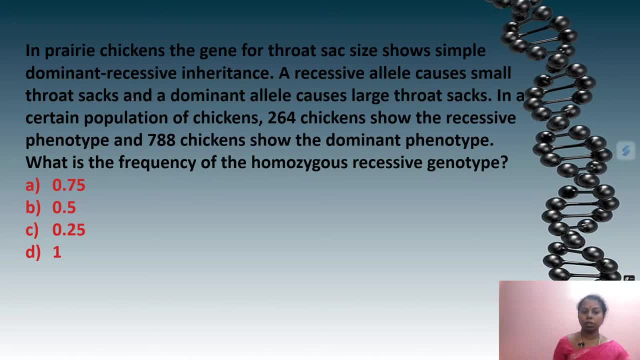 A recessive allele cause small throat sac and a dominant allele cause large throat sacs In a certain population of chicken. 264 show recessive, 788 show dominant. What is the frequency of homozygous recessive factor? Homozygous recessive phenotype? 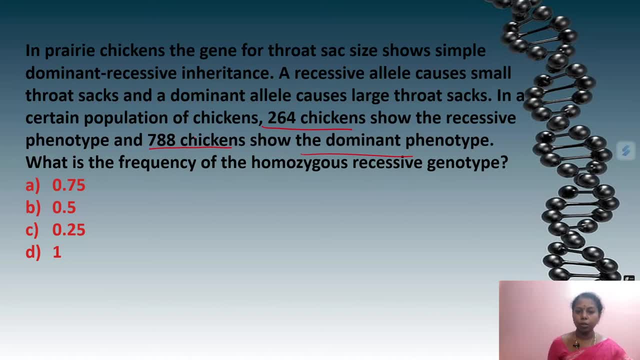 The trick is in the answer itself. If you find out the ratio of 264 and 788,, you can easily find out what is dominant and what is recessive. So what does the ratio of 788 and 264 tell you? If you find that out, the answer is with you. 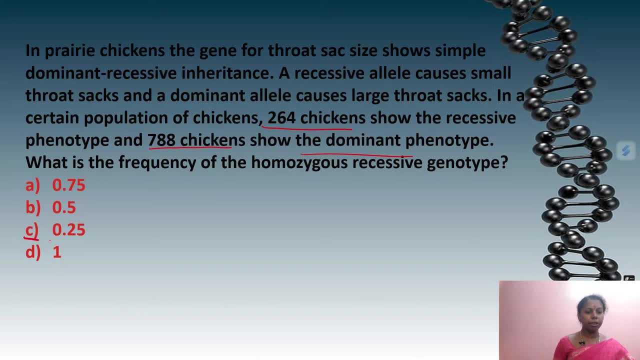 Yes, Tarunika answered C. Excellent, Tarunika, Very good, You are rocking today, Very good. So you know, I told you 788 is 3 and 264 is 1.. That means mono hybrid cross. So you know, 1 is to 2 is to 1.. So recessive genotype will be 1 ratio, which is 0.25.. 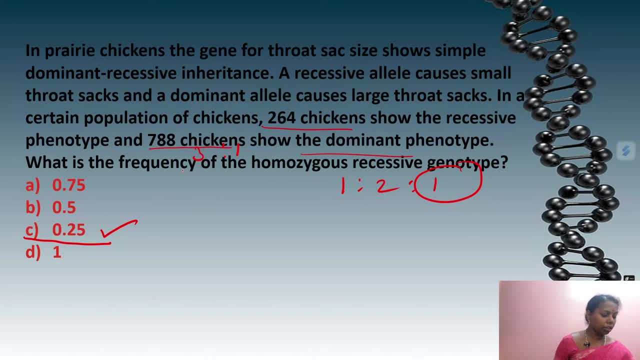 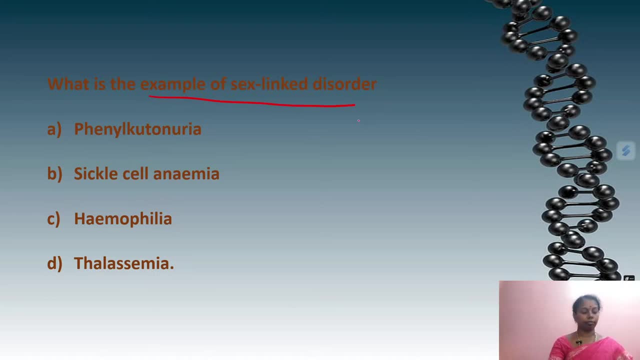 Yes, sir, Very correct. Dharani and Daniel and Santosh Lakshitha- Excellent, You are all rocking. What is an example of sex-linked disorder? Sex-linked disorder? Is it penile ketonuria, sickle cell anemia, hemophilia or thalassemia? 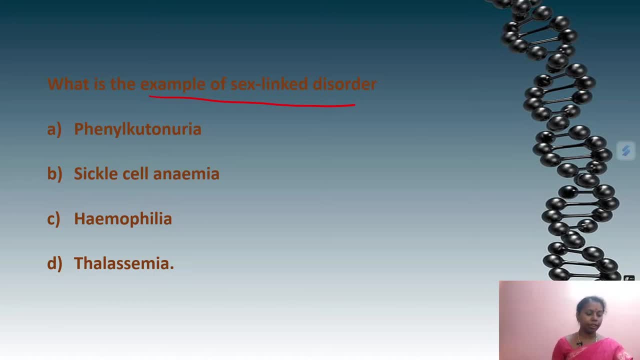 Which is a NCRT theoretical question. It is not application oriented or skilled. Yes, it is hemophilia. Very correct, You know, it is transmitted through sex-linked inheritance from mother to the son and father to daughter. So this is the sex-linked disorder. 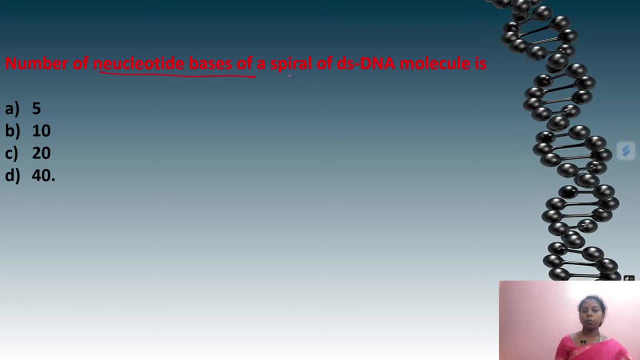 Number of nucleotide bases of a spiral double-strand DNA molecule is how many A spiral double-strand? It is a tricky question, but you know. spiral of double-stranded DNA molecule: Yes, it is 20.. Dharanika, you are rocking. It is your day. Very good, Excellent answer. 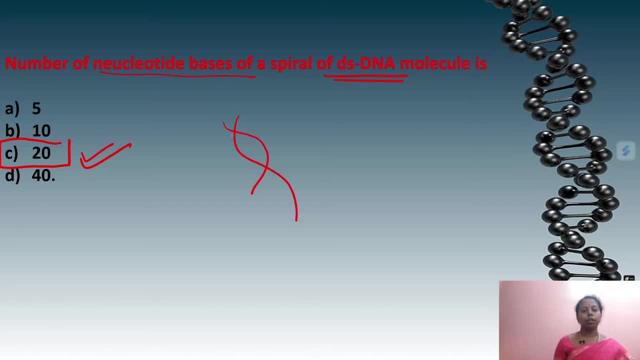 So you know, for a turn you will have only 20 base pairs. no, That is, 10 base pairs will be there. That means 20 nucleotide you will be having in a spiral of double-stranded DNA molecule, So one spiral. we will have 20 nucleotide or 10 base pair. 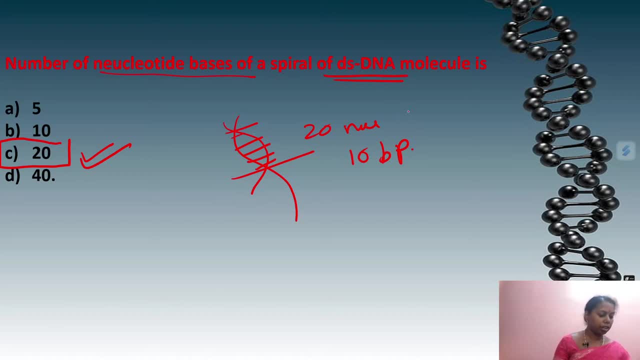 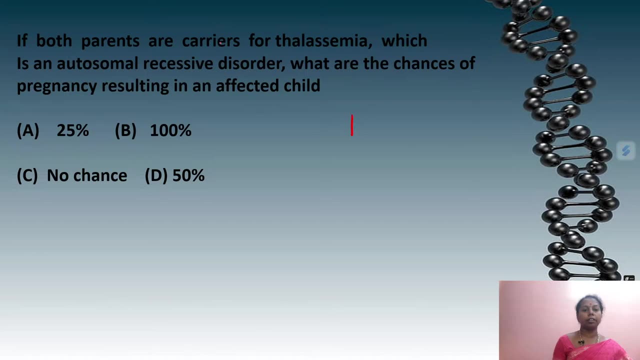 Is the correct answer. Yes, Lakshitha, Daniel Nandika, all of you are correct answer. Now see this question. Both the parents are careful. Both the parents are carriers of thalassemia. So capital T, small t. let me write. 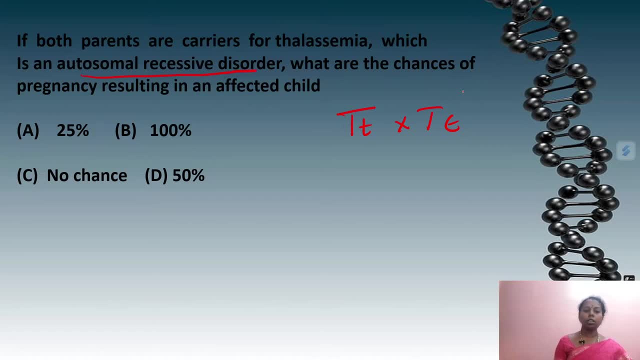 Which is an autosomal recessive disorder. What are the chances of the pregnancy resulting an affected child? So what is the probability for the carrier parents to get the affected child is the question. Please inform any of your friends, Those who are preparing for Meet2024, these questions are really helpful to them. 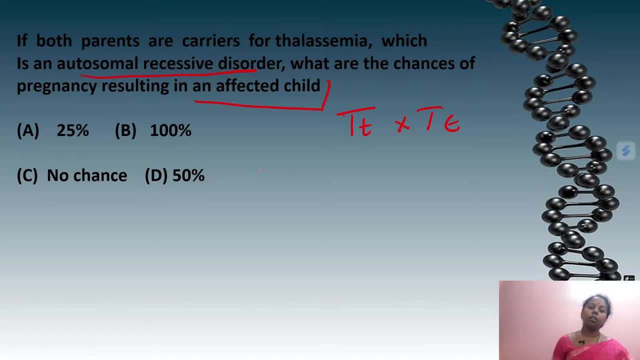 All tricky and application-oriented skill questions. share with them also And any doubtful topic or question, please forward it to me that we can use it for the next live class. It will be more useful for all of your friends. Yes, Dharani, it is A very correct, excellent Lakshitha. 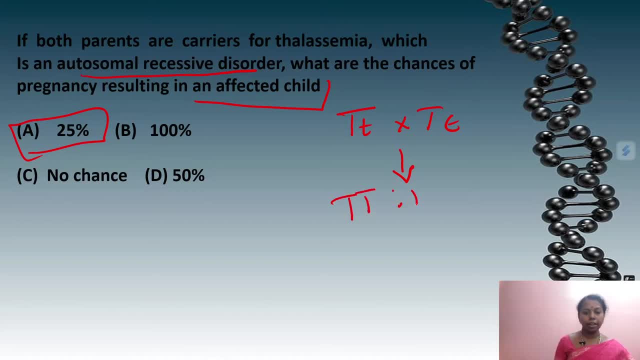 So you know the ratio 1 is to 2 is to 1. Tt, capital T, small t and small t small t are affected. They are asking resulting affected child. Of course it is 25%. Very correct, excellent answer by you all. 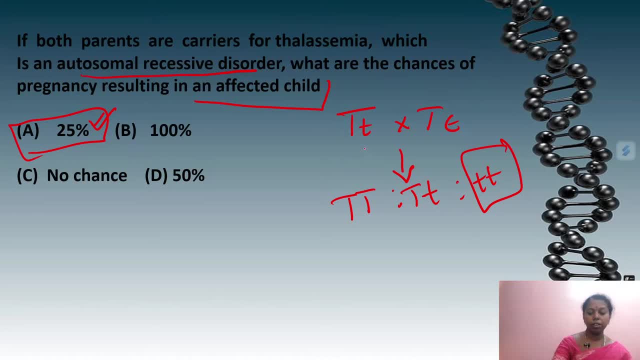 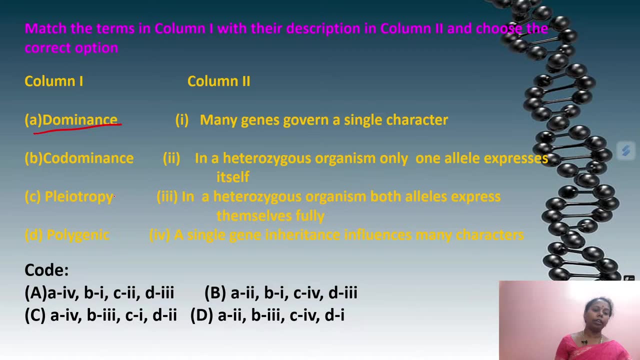 Okay, Yes, Vivekananda and Daniel. excellent answer. Now next question: we have to do the matching. So what is dominant? you know, Yellow seed is dominant, Green pod is dominant, Inflated pod is a dominant. So all these characters are all dominant, right? 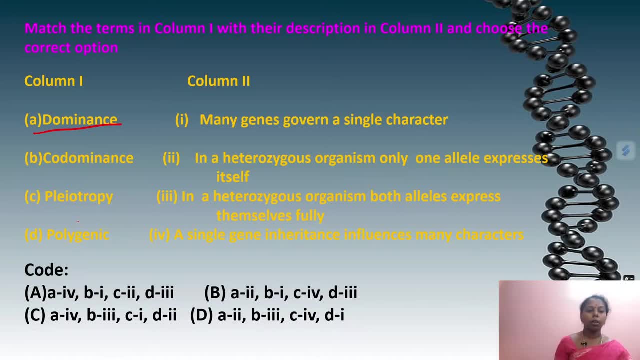 If so, what is it? You will see the explanation. Co-dominant. two characters have come together Now- yellow and red. You will get a character as if both come together. If there is yellow in the petal and red in the petal, that is co-dominant. 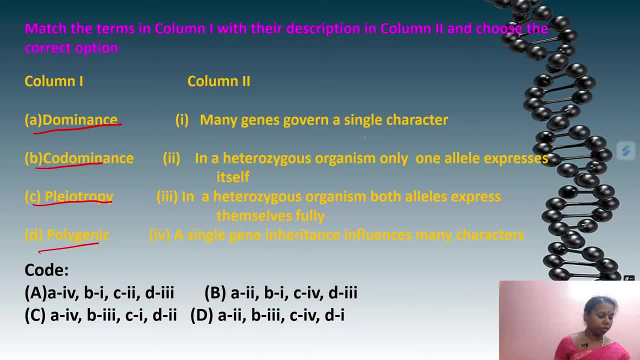 Pleiotropism and polygenic. Have you matched? Yes, Daniel answered Dominance. what he says is: In heterozygous organism, only one allele express itself. Very correct, excellent Co-dominant. In heterozygous organism, both allele express themselves. 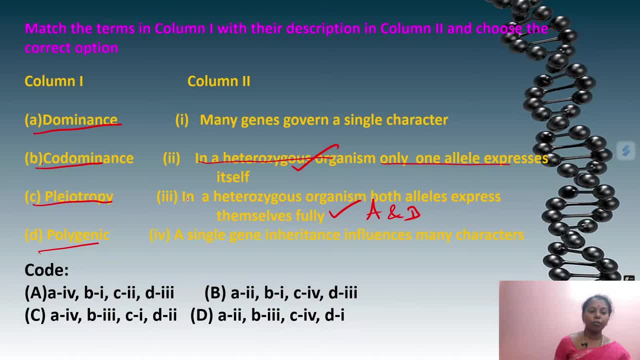 Very good, AO express and PO express. And pleiotropy means what? Yes, single gene inheritance, many character, Is very correct. excellent That also. And polygene- poly means many, Many gene governing single character. Yes, it is D option. 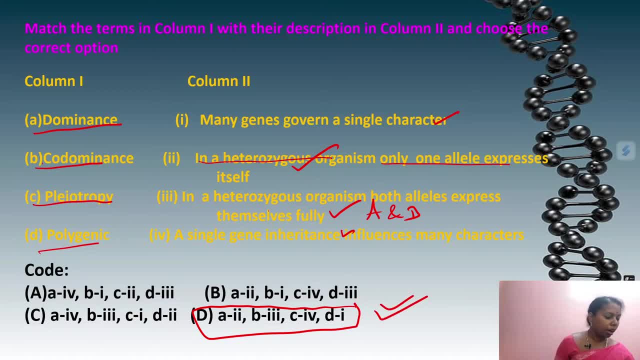 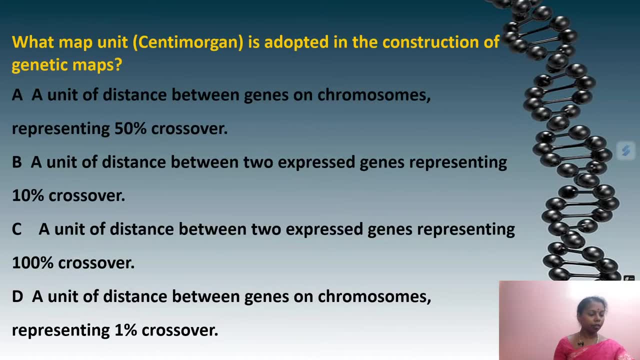 Very correct. excellent, Daniel, You are rocking superb. And Vivek and Nandika, Santosh, Dharini, Tarunika, Lakshita- Yes, excellent answer by you all. Now next question is NCRT line checking. 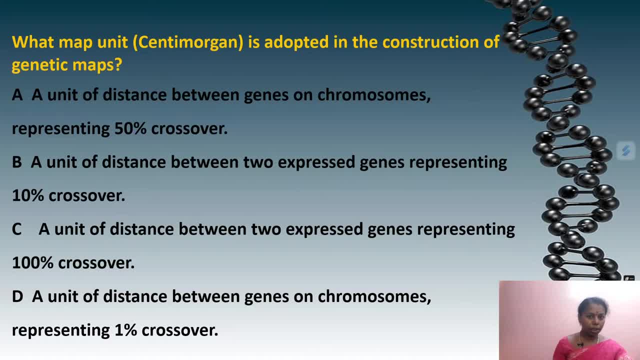 Of course, what map unit is adopted in the construction of genetic map? It is based on 50% crossover or 10% crossover, or 100% crossover or 1% crossover. It is typical NCRT line. Yes, Tarunika, it is 1% crossover. 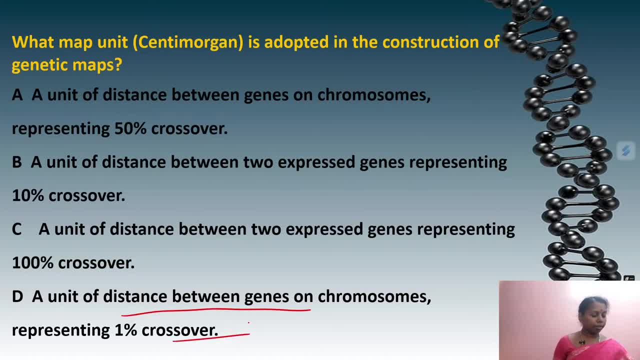 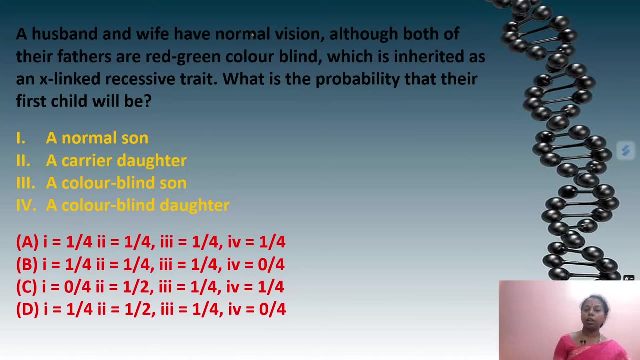 D is the correct answer, of course. Excellent, Nandika and Lakshita. Yes, so it is D. and Dharini? Now this is little tricky question again. Yasmin and Mike: both are having normal vision, But their fathers are having color line. 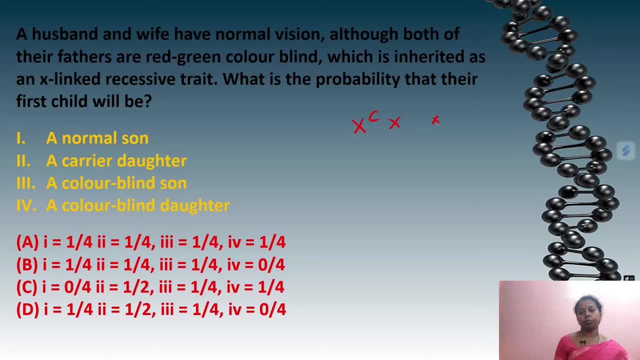 That means mother is a carrier Crossed with XY. No, he is not affected. So father is not affected, because father only father's father only affected. What is the probability of the first child will be having a normal son, carrier daughter, a color blind son, a color blind daughter? 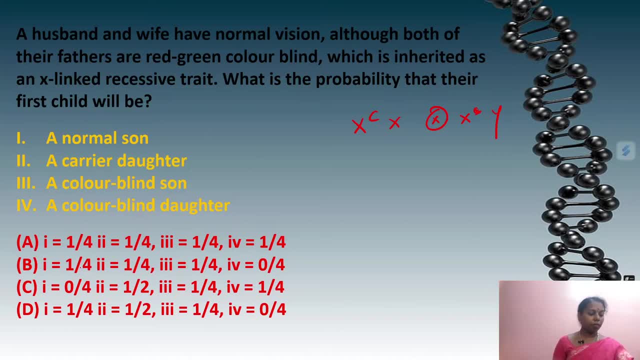 Yes, Daniel, it was D for the previous one. Very correct answer. Excellent answer by you, Daniel. 100%, you are correct. Now next question: We are crossing XCX into X and Y, For your reference. Yes, Tarunika answered. 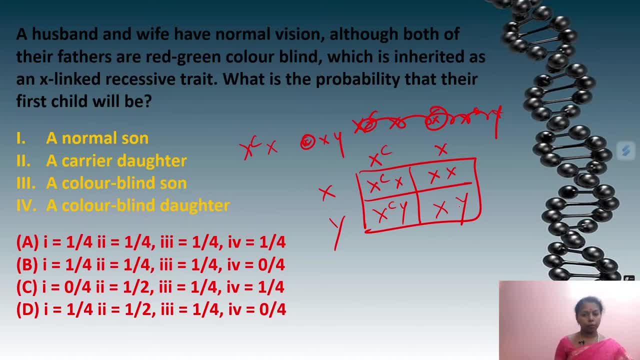 So having a normal son, X and Y is among the 4, 1.. So 1 by 4 is correct. A carrier daughter among the 4.. XCX, 1 by 4 is correct. A color blind son Among the 4 is 1.. 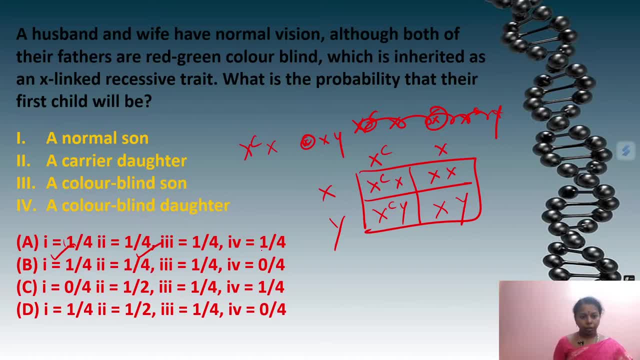 XCY. Okay, So again that also 1 by 4.. Now, color blind daughter. we are not having XCX, we do not have. So 04 is the correct answer. It is B. Very correct, Daniel and Tarunika. 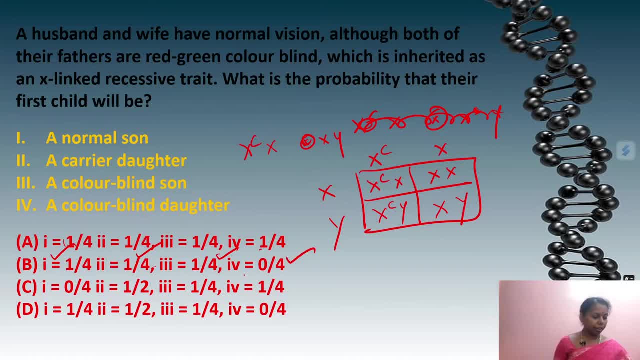 Excellent answer by you. Both of you Very correct. Now this question seems to be tricky, But it is answer is very easy, Try. Yes, Nandika, It was B for the previous one. Yes, Tarunika, Excellent answer by you. 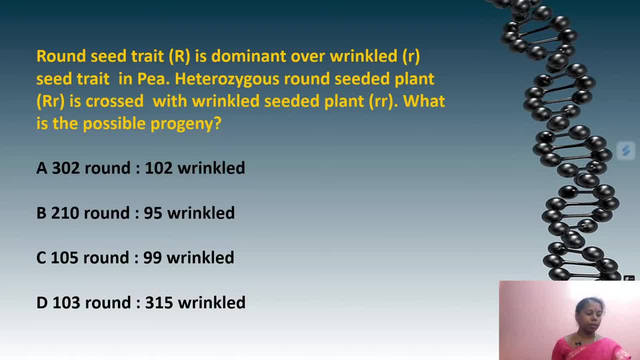 Both of you Very correct. Now this question seems to be tricky, But it is answer is very easy, Try. Yes, Nandika, It was B for the previous one. Yes, Tarunika. Excellent answer by you, Both of you. 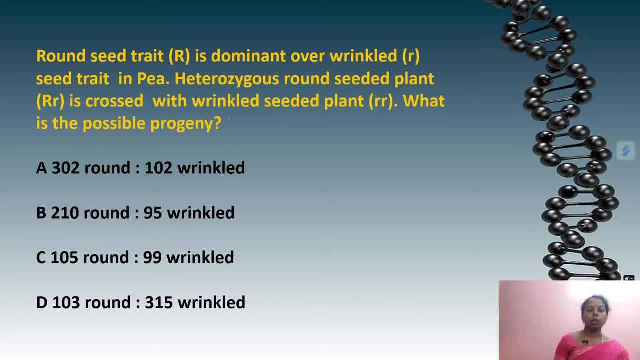 Yes, Tarunika, Excellent answer by you, Both of you. Now, round seed tribe is dominant over wrinkled. in P Etrozygous round seed plant is crossed with wrinkled seeded plant. What is the possible progeny? See Etrozygous capital R, small r. 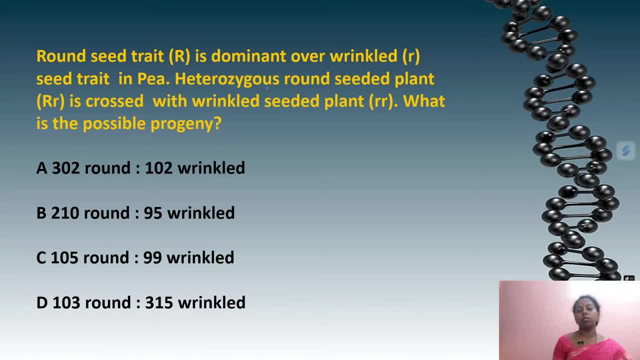 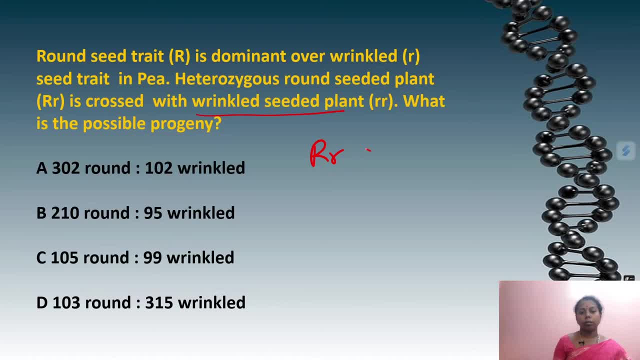 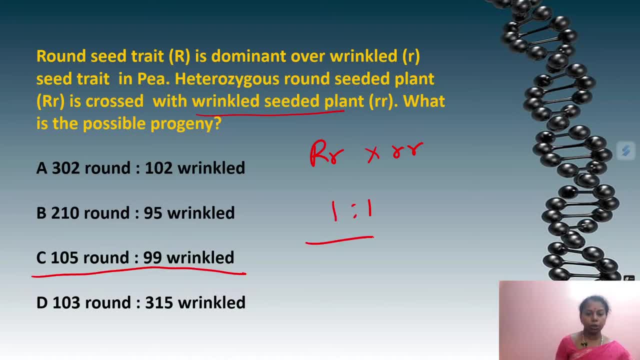 Yes, it is C. If you see, 1 is to 1 is the ratio. Okay, So almost here we are getting around 100, both the values. So 1 is to 1.. C is the correct answer. Excellent answer by you all. 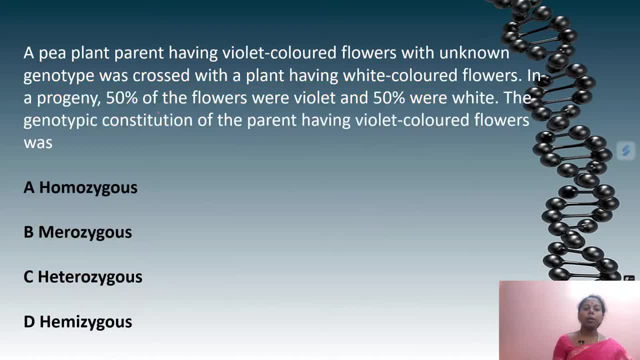 Now next question. Let us see A pea plant parent having wild plants. Violet colored flower with unknown genotype was crossed with a plant having white colored flower In the progeny. 50% of them are violet. So 50% violet and 50% were white. 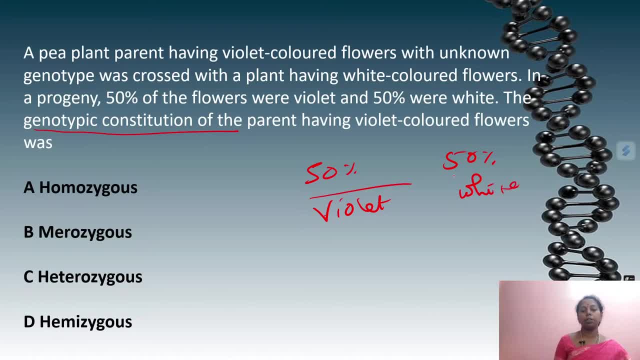 So what is the genotype constitution when we get 50%? 50% is the question. Yes, Dharanika, it is heterozygous. Very correct, Excellent answer. Yes, Daniel, Of course, heterozygous, only we will get this sort of arrangement: 50 and 50. 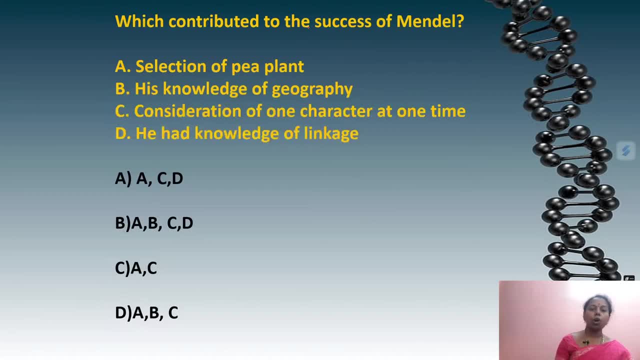 Yes, Okay. Now next question, Which contributed the success of Mendel. So Mendel was succeeded For so many reasons. It was the first introduction in principle of inheritance, So what was the points which made him very much successful? 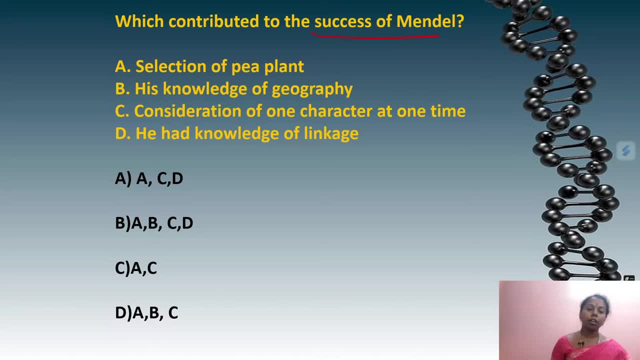 Of course, he was very using implementing statistics and mathematics in biology, which is not mentioned here. anyway, I am telling you, And he was the first person to use the word factor for the gene. So all that are contribution Like among this. 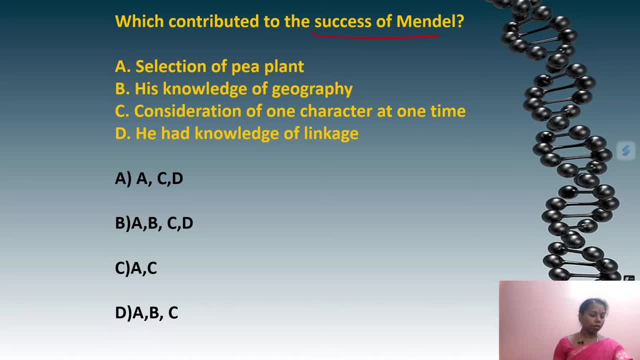 What is listed here? What are the contribution is the question. So Vivekanth, and already answered, Daniel answered: Yes, it is A and C. Very good children, You are okay. Yes, Selection of P plan, because you know various reasons: self-pollination, cross-pollination. 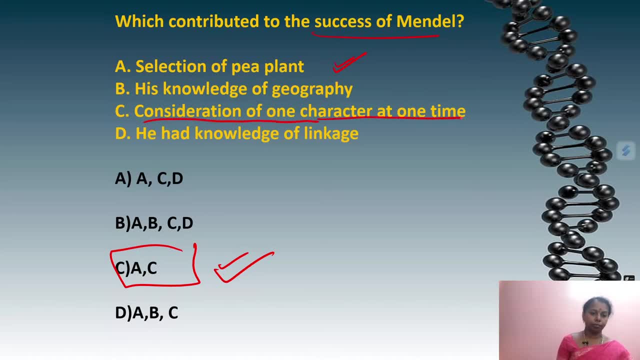 all that One character at a time. He does not have any knowledge on geography and knowledge of linkage, So that he made independent assortment and all, Of course, these two A and C is the contribution. Correct answer: Lakshita Dharini, Nandika, Tarunika and Daniel. 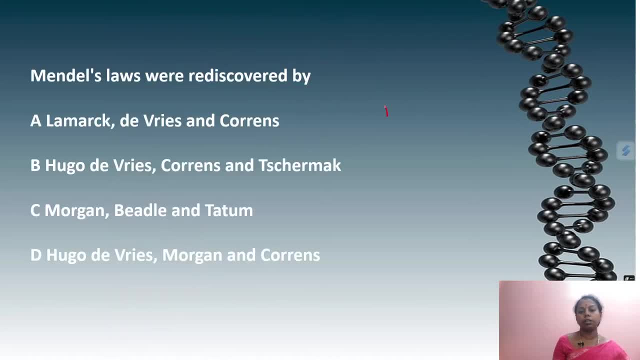 Excellent answer. Mendel's law were rediscovered. It is typical NCRT line. Who are those scientists who worked on Mendel and reworked and find out? it is correct, And after 19th century only we named him father of genetics? 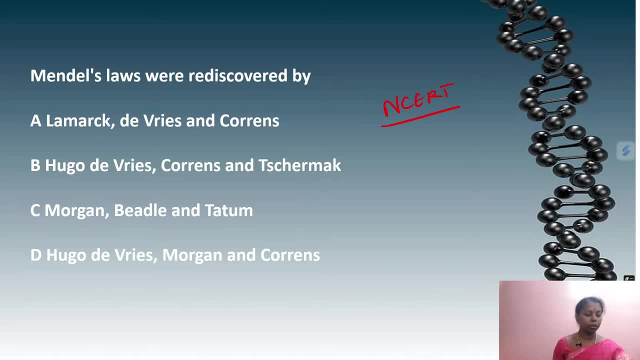 But poor man, he does not know that he is the father of genetics. He is no more that time. Yes, Yes, who are those three scientists? Very easy NCRT line. Yes, it is we: Hugo DeVries, Car and Santesh Sharma. 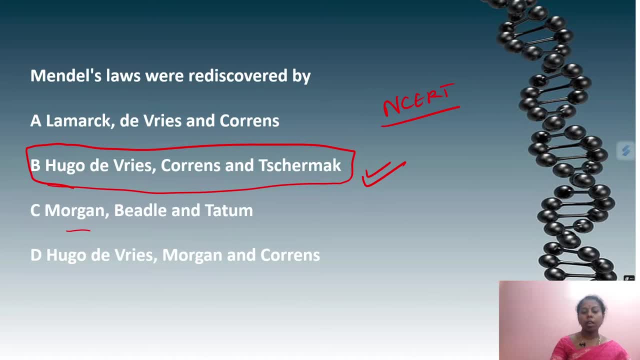 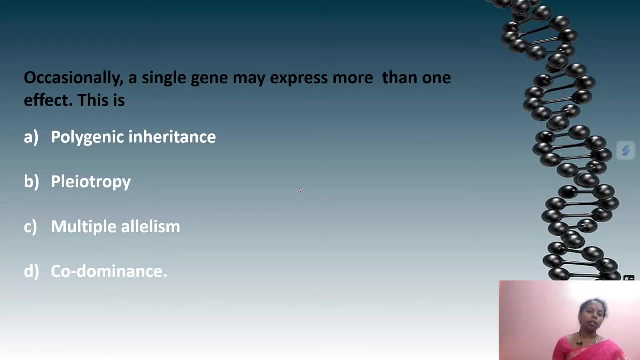 Or those three scientists who work. Yes, Daniel, excellent answer. and reworked on Mendel's concept and said whatever he said is correct. only, Okay, A single gene has more than one effect. that is called dash. So one gene control many character. 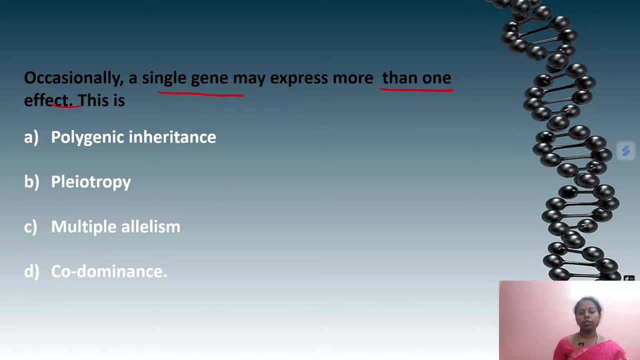 A single gene control many character. A length of the wings in Drosophila, number of goba produce. So all these characters are controlled by one gene. means the character is called dash. Yes, excellent answer by Daniel. It is pleiotrophism. 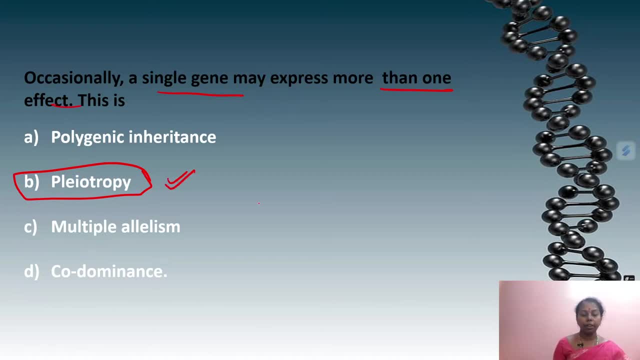 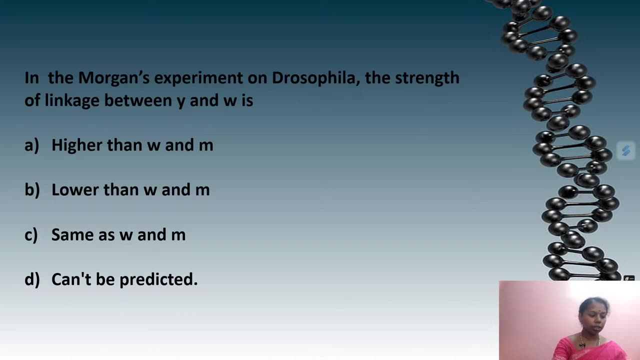 Pleiotrophism, where one single gene is controlling many character. Yes, it is pleiotrophy, very correct. Okay, This is a tricky question, but NCRT, only In the Morgan's experiment on Drosophila the strength of linkage between Y and W is: